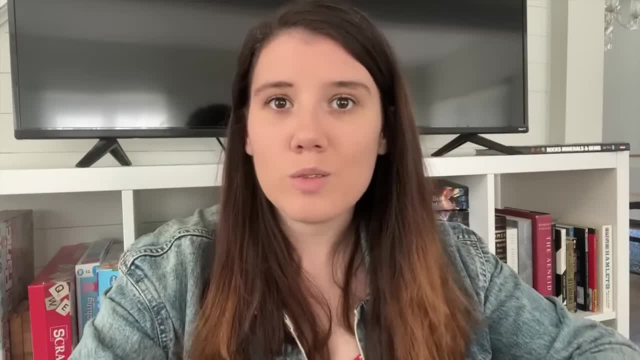 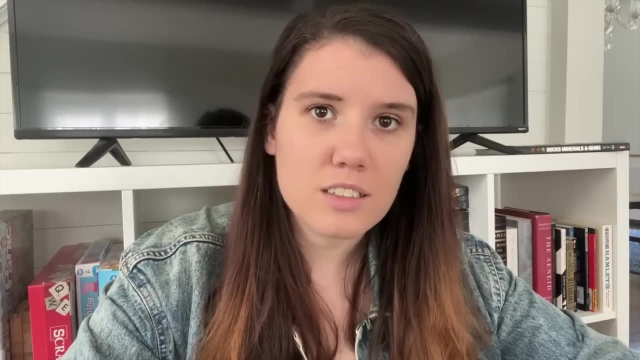 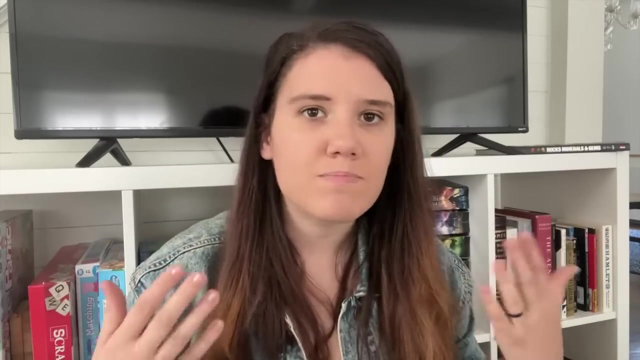 A crackpot will then send this theory to a physicist and demand a response, but really they're demanding praise for being a physics genius. there are exactly two types of crackpots. type a is the retired engineer, like someone who worked in a science adjacent field, like maybe when they 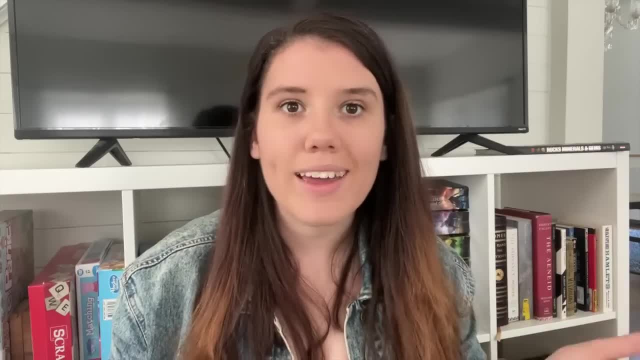 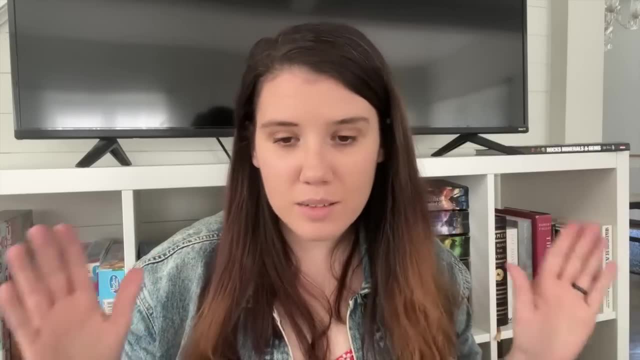 started college, they wanted to study physics, but life got in the way, and now that they are retired, they finally have the time to dedicate to their passion, and i think that's amazing. i admire that so much, but the problem is that instead of maybe watching some con academy videos or to 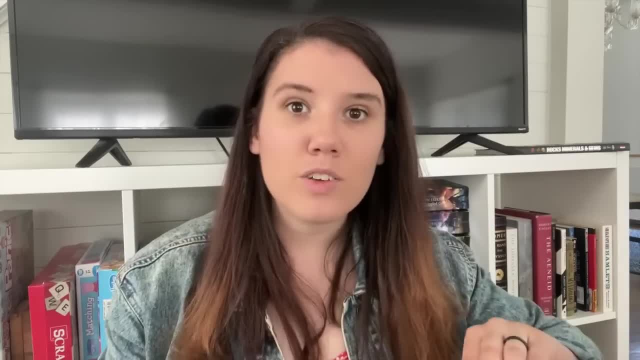 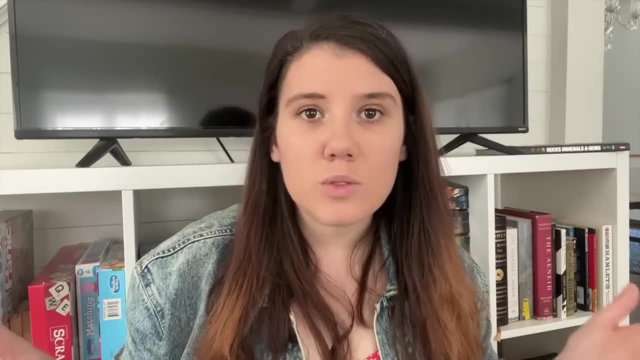 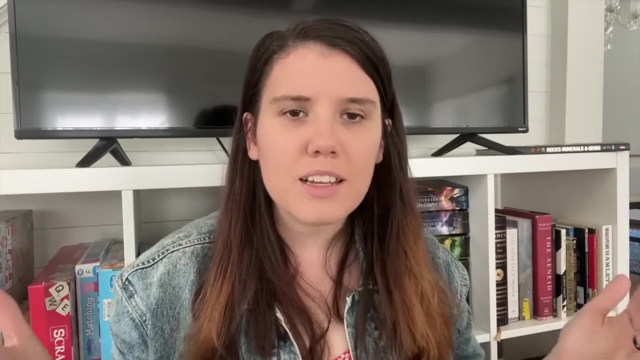 making an entry-level physics course. they jump just head first into whatever topic's been fascinating them for the past 30 years. so like i'm gonna pull out a graduate level textbook on general relativity or the latest paper on dark energy or string theory and immediately they're 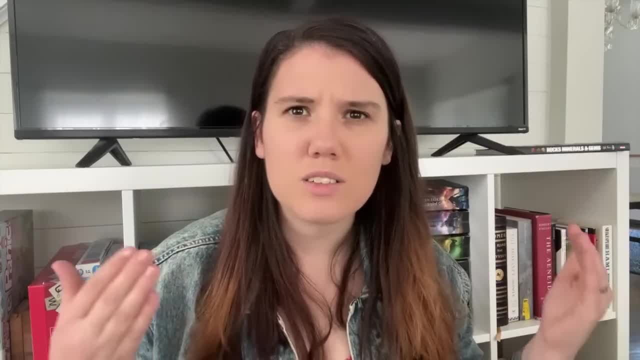 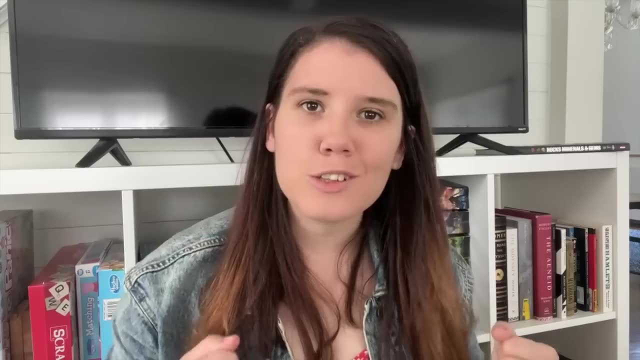 completely lost. so they're like: this doesn't make sense to me at all. this isn't what i thought physics would be like, and instead of like chuckling to themselves and saying i should get back to physics to get started and spending the time to build up that background, the crackpot kind of. 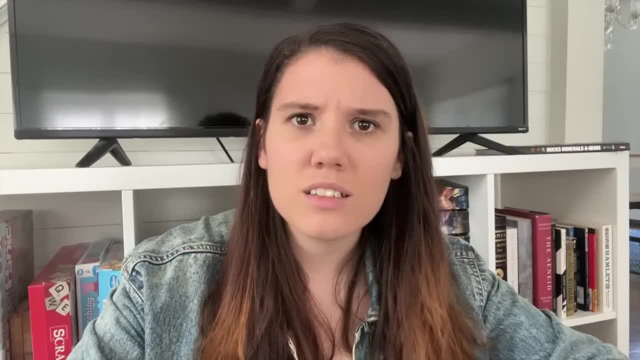 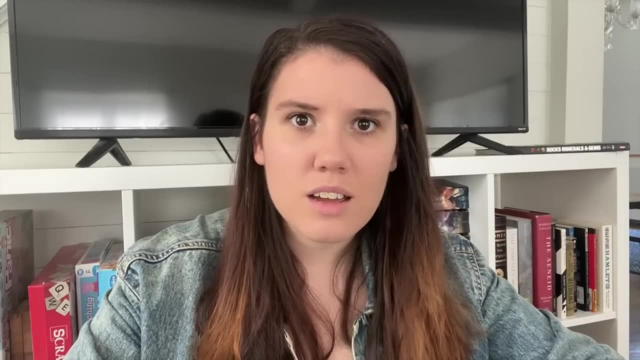 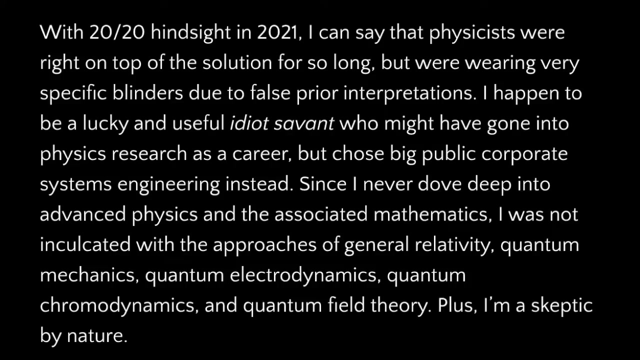 responds like i don't understand this at all. this must be wrong. physicists are wrong. i'm gonna start writing my own theories here. here is an example i found on a crackpot's website. to kind of highlight this personality, i can say that physicists were right on top of the solution for so long, but were 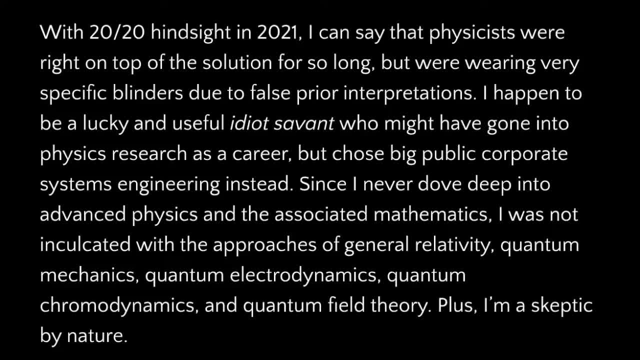 wearing very specific blinders due to false prior interpretations. i happen to be lucky and you can't tell- but i've been lucky enough to have a good friend of mine who's a very smart and useful idiot savant who might have gone into physics research as a career but chose big public. 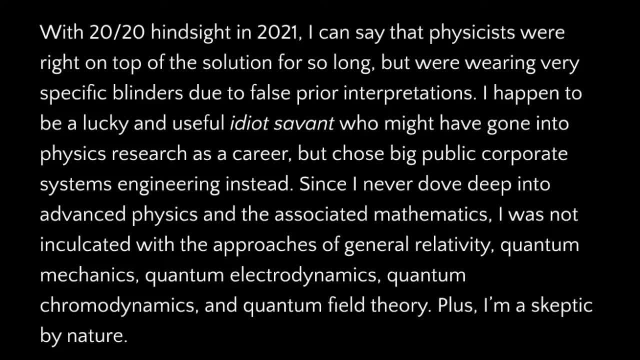 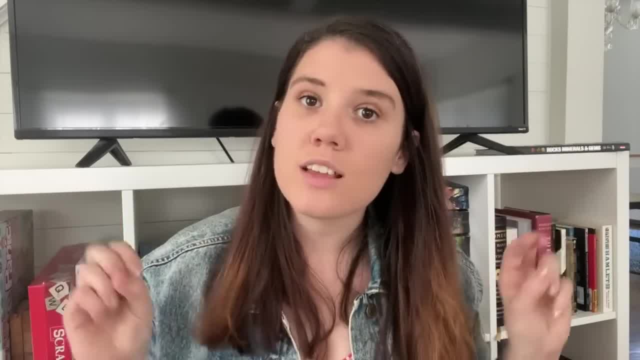 corporate systems engineering instead. since i never dove deep into advanced physics and the associated mathematics, i was not inculcated with the approaches. so at this point they've decided that physicists are wrong and they're going to be working on their own theories, and they never go. 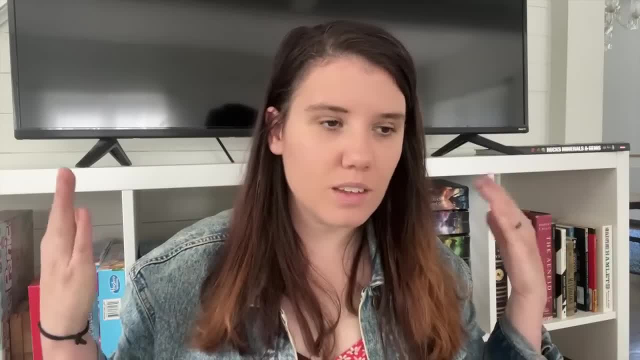 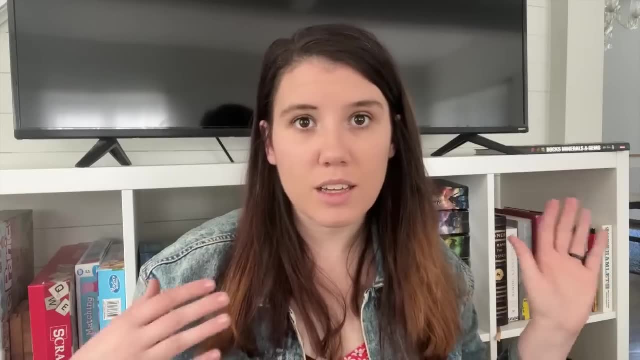 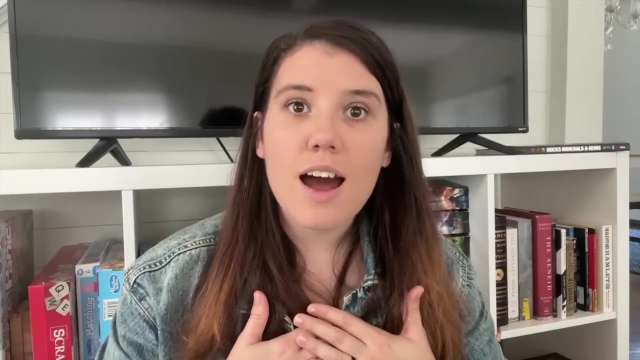 back to learn the math. type b is very similar. i'm going to call it the dropout. so it's a smart person, probably enjoying popular science, media related to physics, like michio kaku books and the big bang theory, and he goes to college and he's like: i'm a smart person, i'm gonna do physics, i'm gonna help. 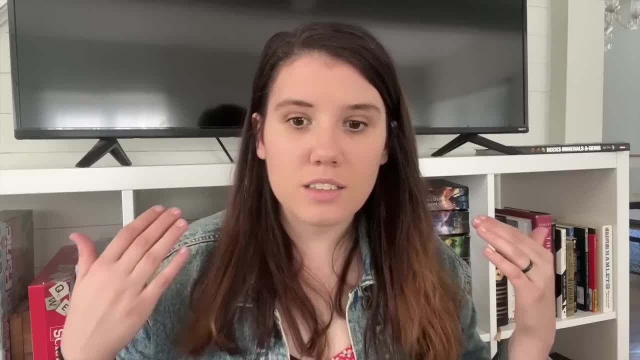 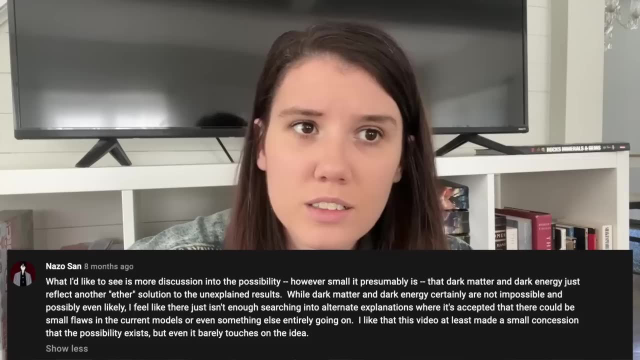 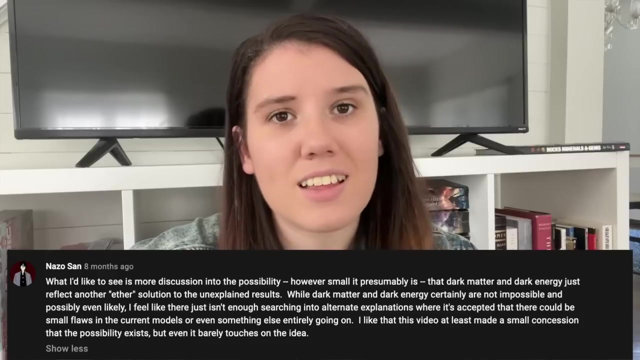 the world with my smartness and my physicsness. and he doesn't do that well, so he will go to the ta's office and be like: i don't understand. i'm smart, physics is innate. i should be good at physics. i understand the physics, i just don't understand the math, and that's. 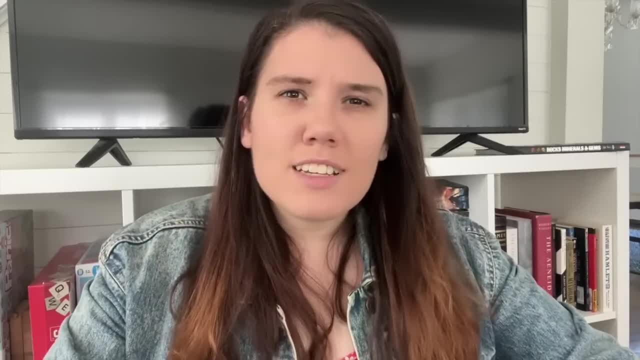 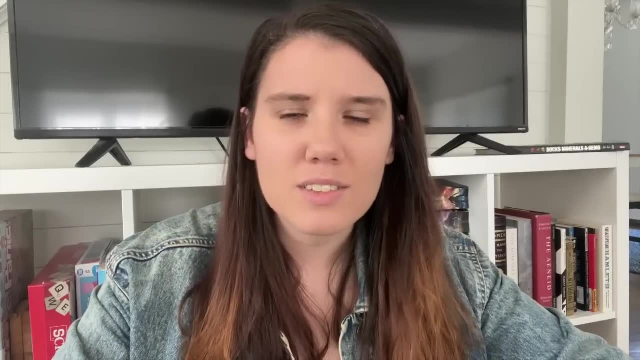 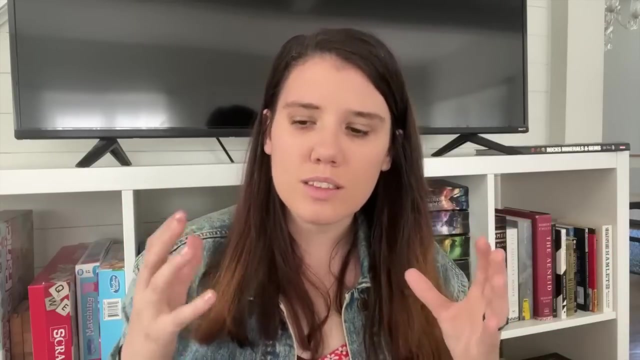 why i failed the test, which is very funny. um, you can't do physics without math. when you say i understand the physics but not the math, you're kind of saying: you understand physics the way a baby understands physics, like a baby in a high chair holding a ball- knows that when she throws 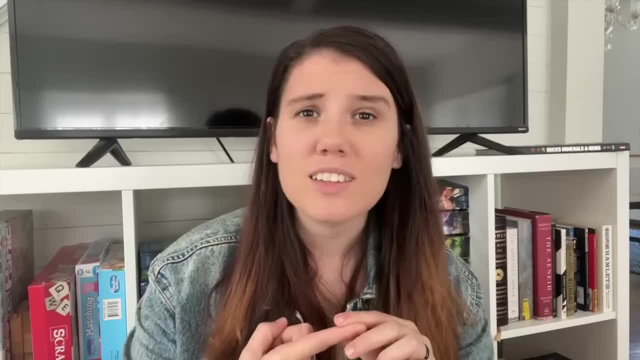 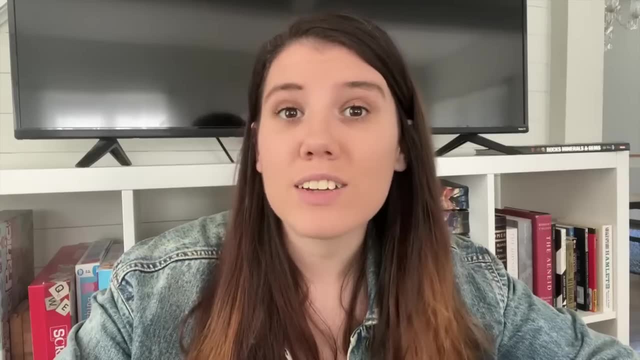 that ball, two things are gonna happen: it's gonna kill, everyone's gonna laugh, they're gonna love it and to the ball will hit the ground. that baby does not know physics. that baby does not know what the word gravity means, but she understands physics without understanding the math. but that is not doing academic physics. 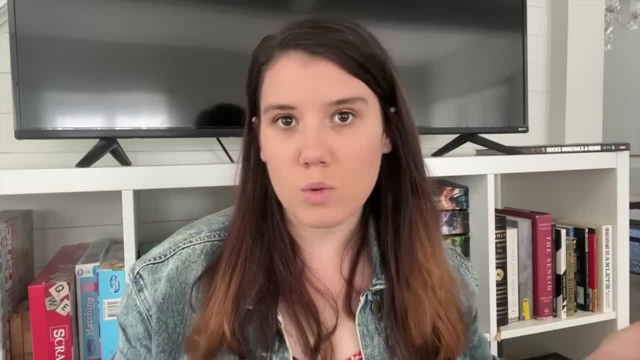 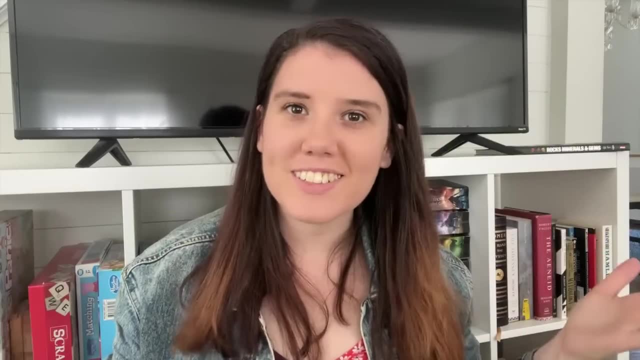 that is not doing physics research, that is just living in the world and having a body and experiencing the worlds. so our dropout tries to convince the teacher how good they are at physics and they're unsuccessful because they don't take the time to learn math, which is very 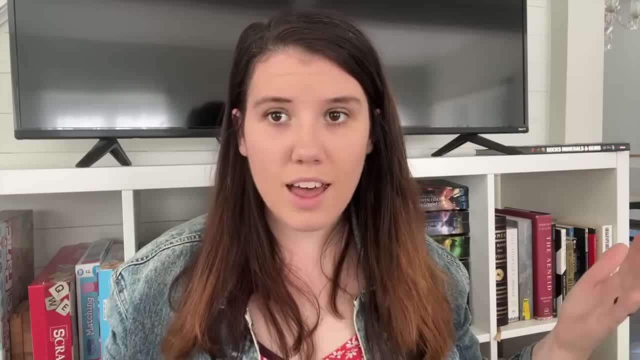 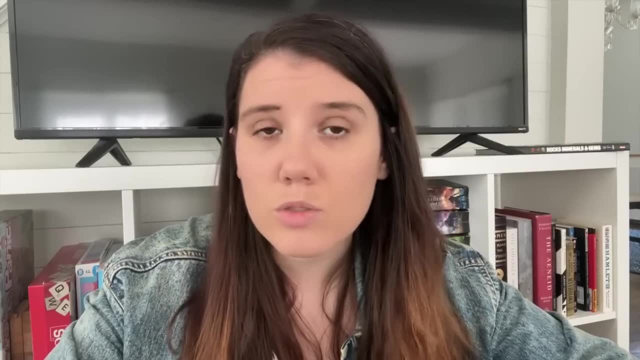 common with crackpots and they fail the course. and that is when they decide there's something wrong. there's something wrong with physics. there's something wrong with the way physics is taught. there's something wrong with the professors. i am smart. i should be good at physics. there's 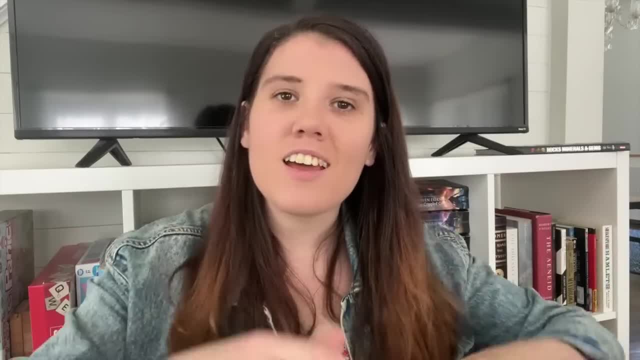 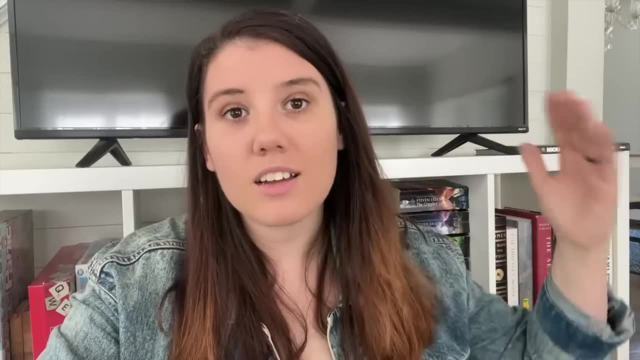 something wrong and they start developing a theory physics. a perfect example of that i found recently on nate silver's twitter. now, i'm not saying nate silver is a physics crackpot, he is an economist. but he tweeted this and it just encapsulates that attitude perfectly. 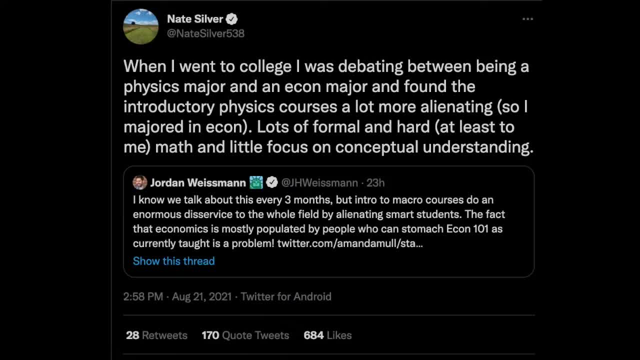 when i went to college i was debating between being a physics major and an econ major and i found the introductory physics course is a lot more alienating. so i majored in econ: lots of formal and hard- at least to me- math and little focus on conceptual understanding. um, but it's very. 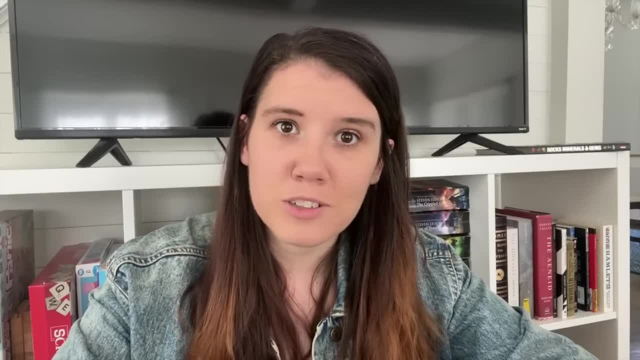 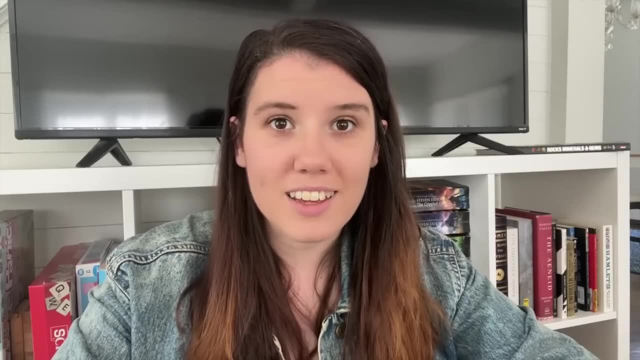 funny to me for two reasons. the first is that nate silver is a professional economist and economics is a hard science. there is a lot of complicated math in economics, like the movie a beautiful mind. john nash is a nobel prize winner in economics and the math looks like this: 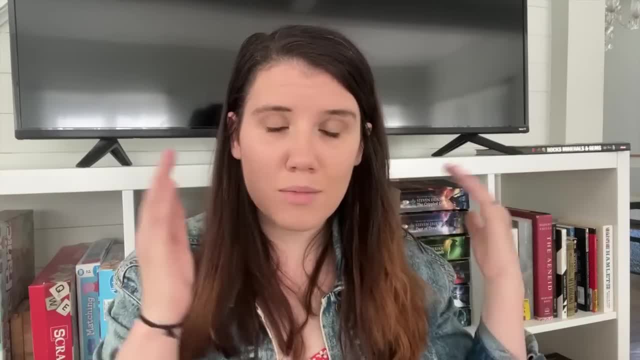 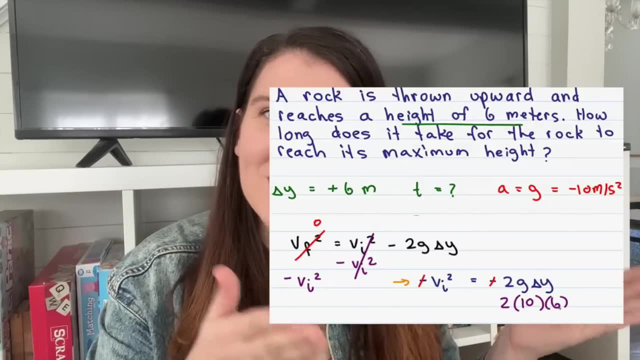 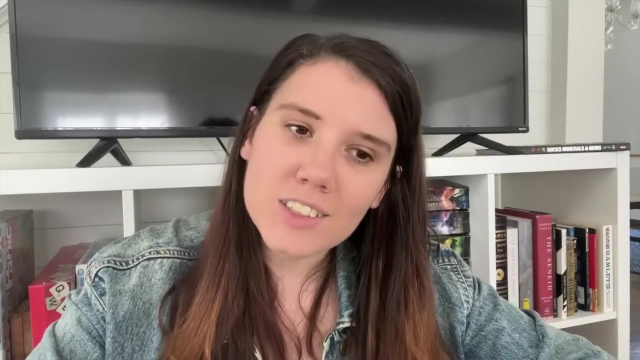 and an entry-level physics course. the math looks like this. i mean, no, math anxiety is real. i'm confident, nate silver, you could have done this math if you just studied at home, if you practiced algebra before going to physics. like why, why do crackpots think that physics should be? 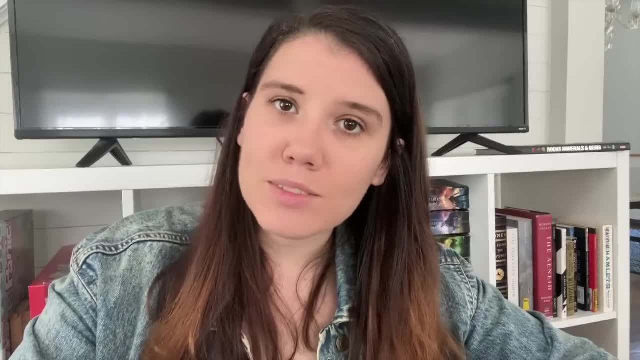 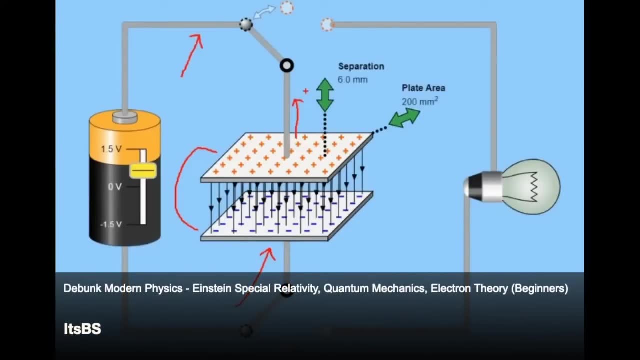 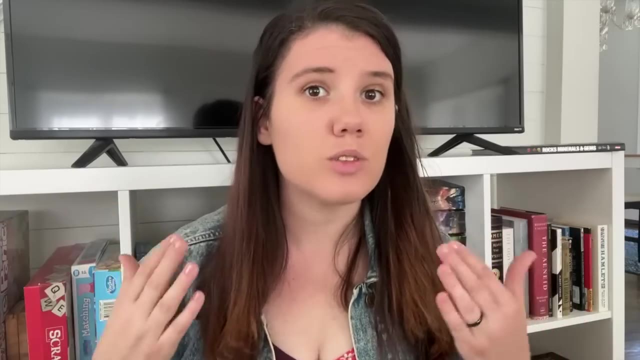 innate and easy. why not take the time to learn the language of physics? the problem with electron theory is it cannot properly describe how a capacitor works. so we have our crackpot boys. they have different backgrounds, but their attitude towards physics is very, very similar. they expect physics to be innate. 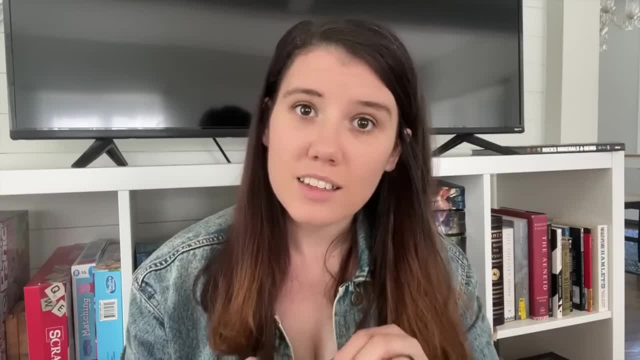 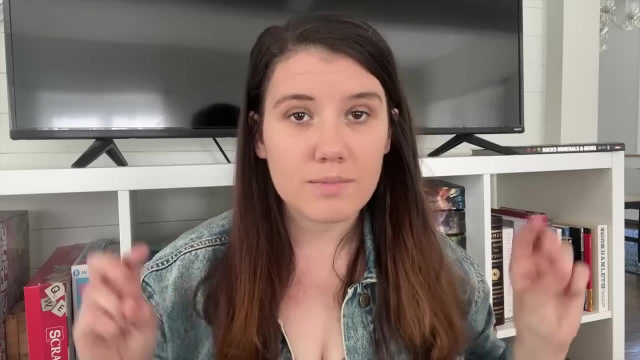 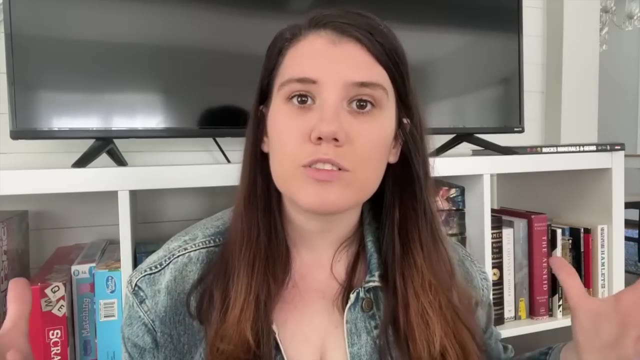 they are smart, they should be able to get it. the fact that they cannot understand a physicist paper on first read means that there is a problem and their theory theories will be better. even though they haven't worked in physics, even though they don't know the language of physics, they don't know the math, they will produce a theory of phys. 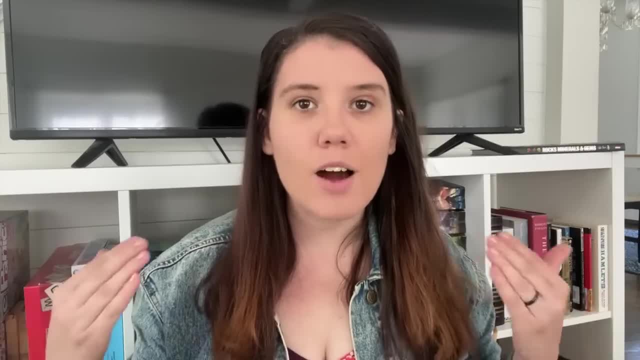 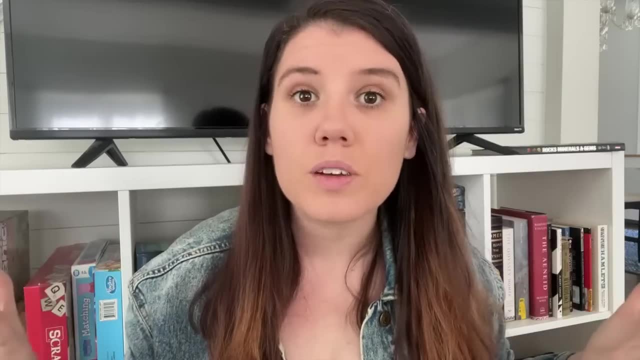 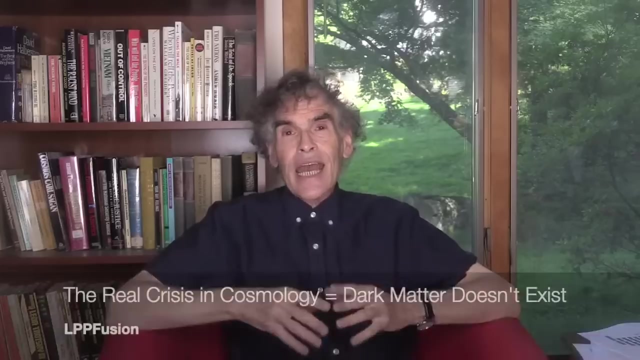 a theory of physics, a paradigm shift in how we think about the world and the fact that they don't have a physics education, they don't have a physics background. it's a. it's a, it's a boon, it's going to help them. they are a gift to the world and we just have to listen how cosmic evolution happened. 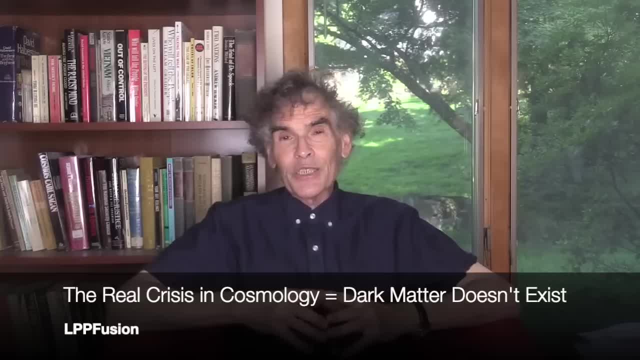 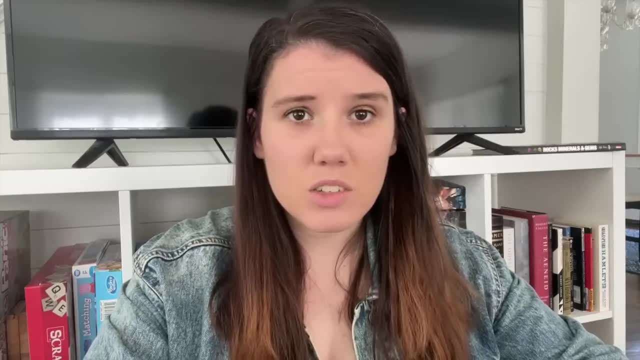 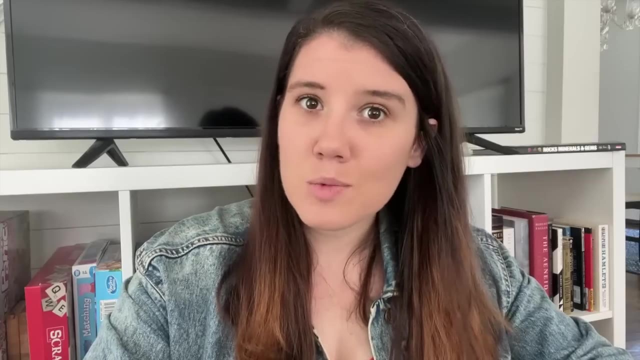 with no big band, no dark energy, no dark matter, nothing dark at all. i have been a physicist for the past 20 years, but i'm not sure i'm a physicist. you don't know me, you don't know what my work is. i probably receive 30 or 40 crackpot emails a year. 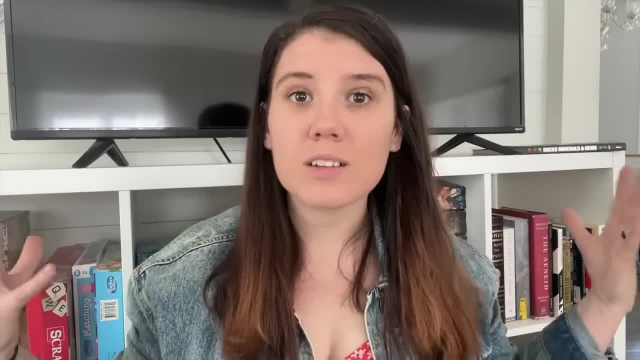 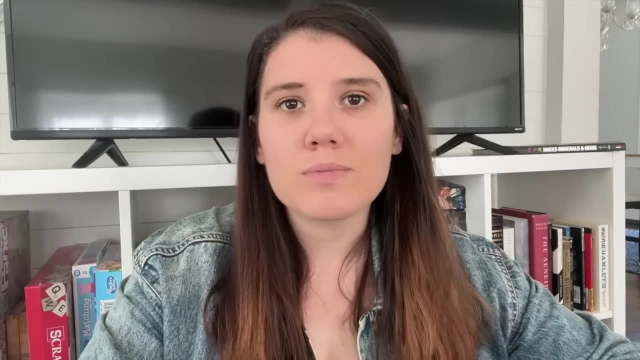 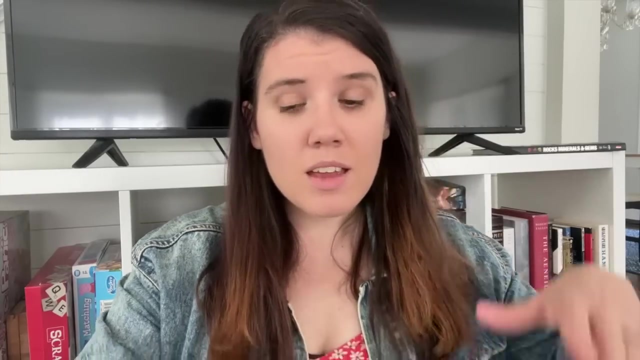 and as a woman i receive way less than my male colleagues have like a similar career level, which is interesting- crackpots. but i can't imagine how many emails well his secretary, how many emails kip thorne's secretary receives from a thousand crackpots a year maybe. 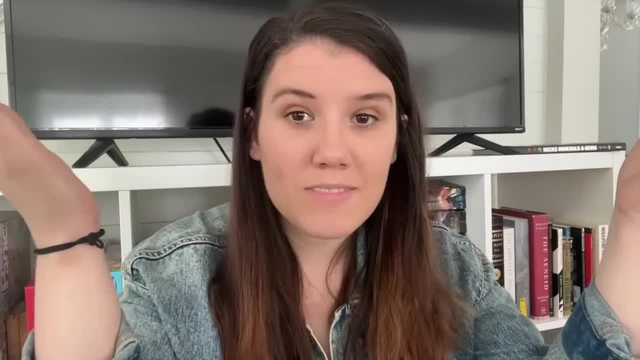 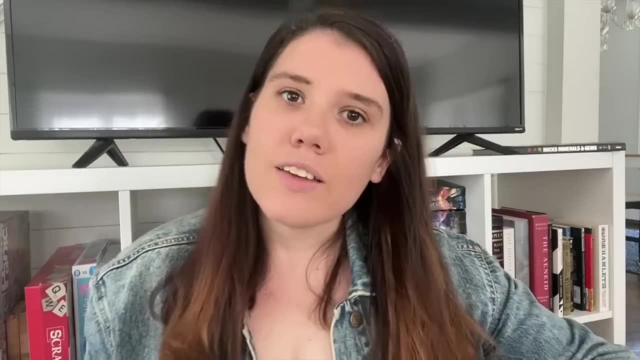 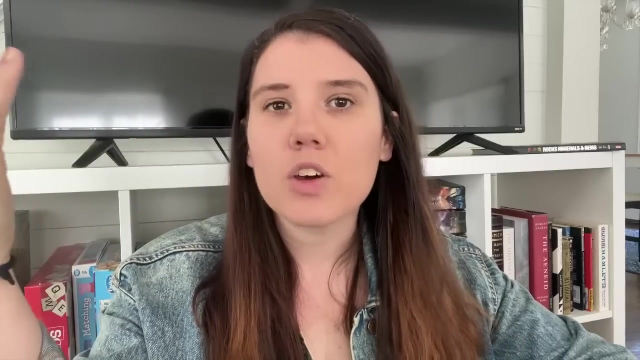 all of these theories are identical and this phenomena of individual crackpots writing identical theories of physics has been known for a super long time. If you google crackpot physics, this list will come up and it's kind of just like a quiz, like a checklist, like a bingo card. 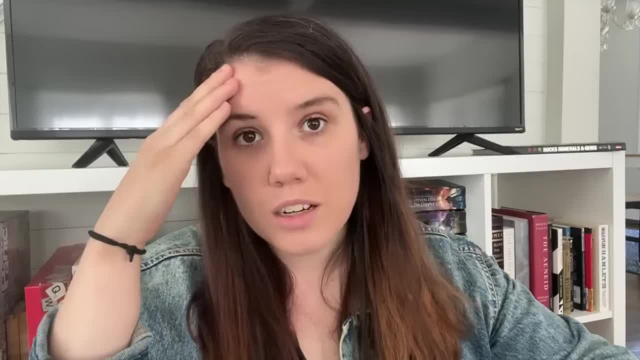 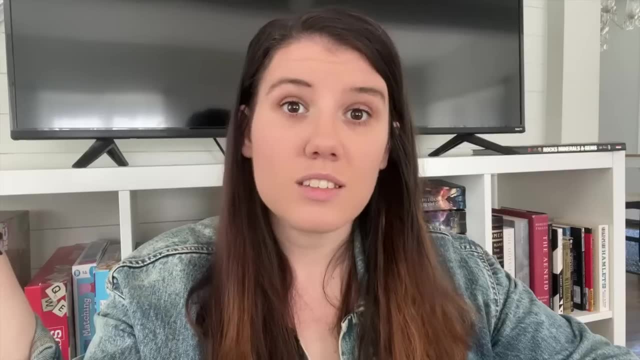 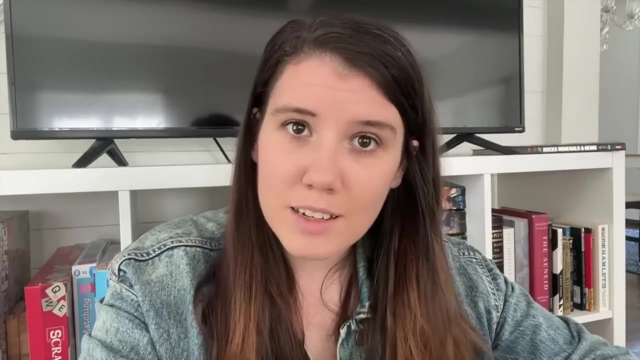 for crackpot theories of physics because again, they are so similar and this is from the 90s. Crackpot physicists have existed for as long as physics has been like a popular science to get into. They used to type their theories and mail them in the physical mail. 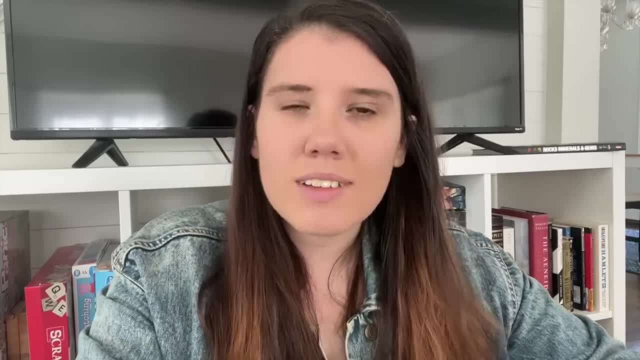 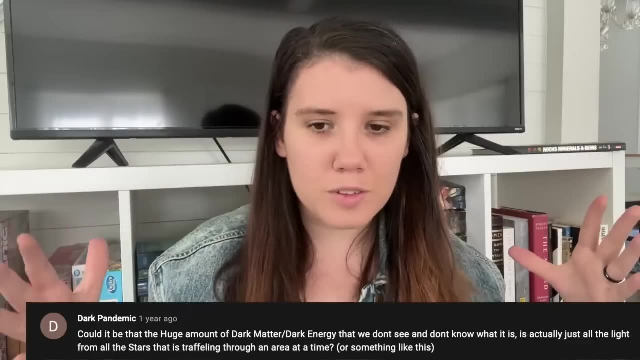 They used to fax them to physics offices. I don't want to go through a crackpot theory and like point out all the bingos I'm more interested in, like the global phenomena, like what makes all of these crackpots come up with the same ideas and 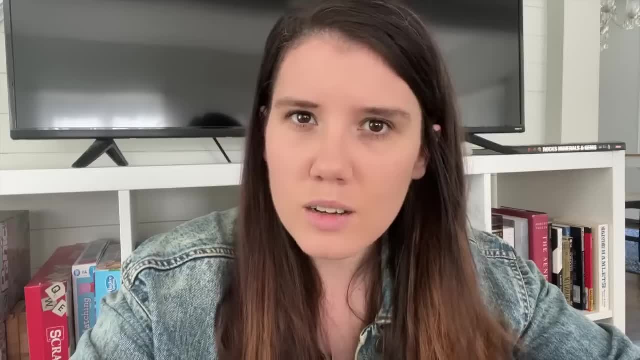 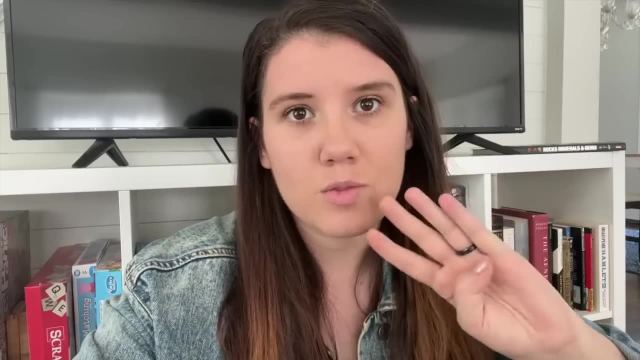 what makes all of these crackpots come up with the same ideas? Why And why won't the physicists respond? What about your emails? No one's responding to your emails. So I just want to talk about four things. Four things that scream crackpot to me when I see them. 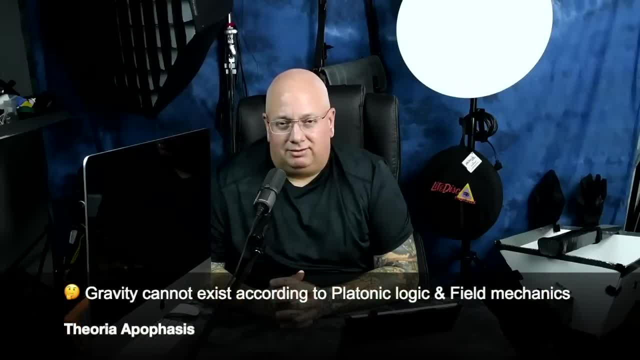 At the center of any supermass there is obviously no gravity. You can take the largest mass in the universe, the center of which obviously you would free float if you could go to the center of it. so where is the center of gravity? The first thing. 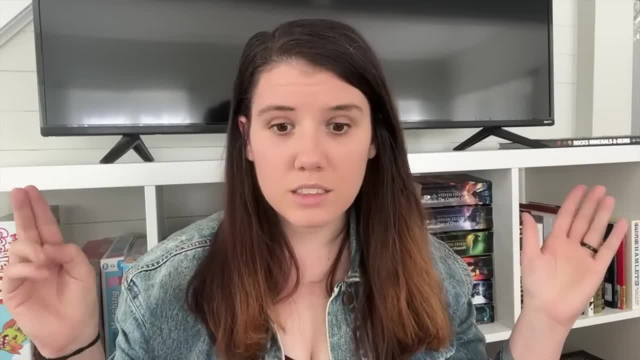 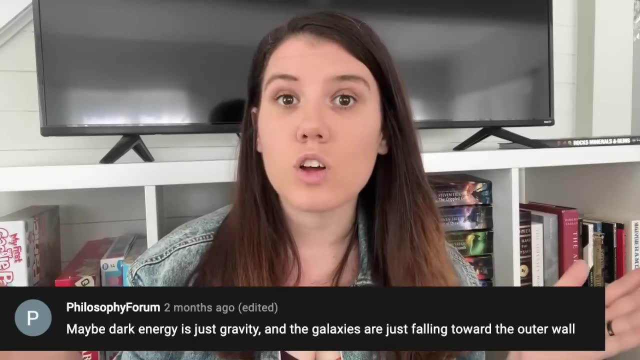 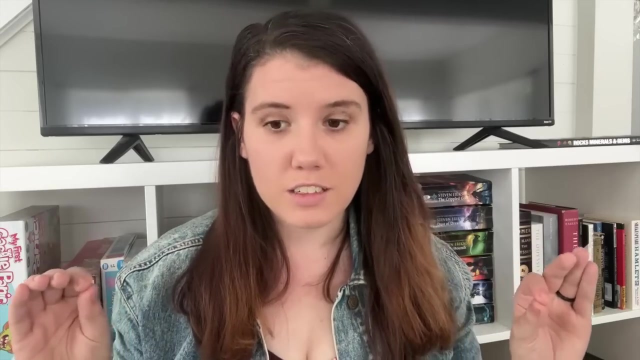 the most emblematic of crackpot theories is that they're always huge- Not in length, but in like concept. A crackpot wants to solve the world's biggest problem. They want to be a paradigm shift in the way we understand physics. They will prove that quantum mechanics is wrong. They will prove gravity doesn't exist. 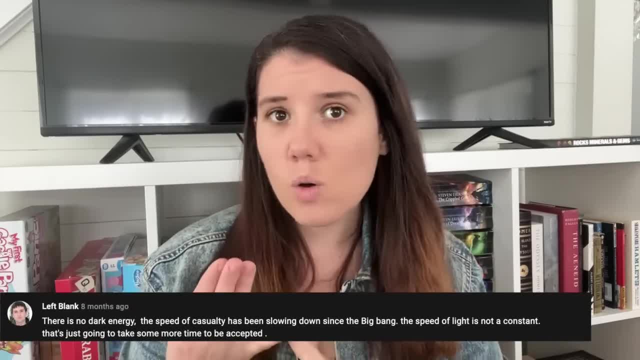 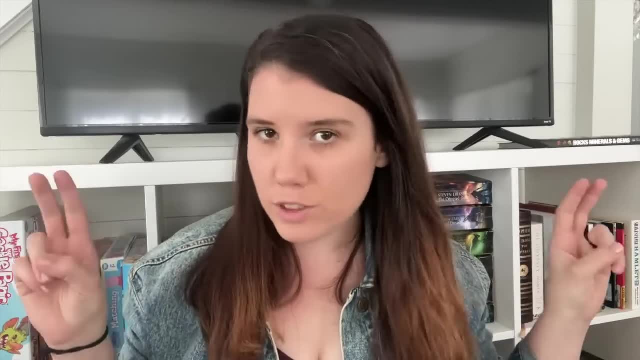 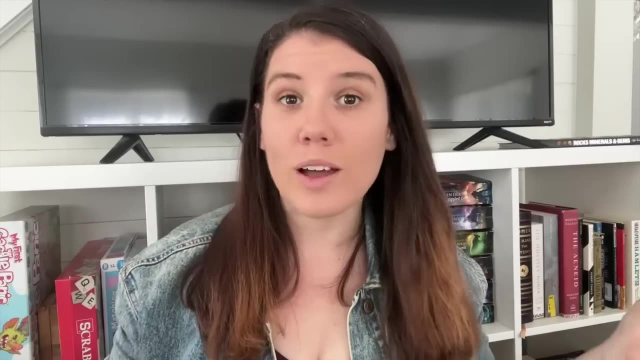 They will prove that electrons aren't real, black holes aren't real, just the hugest things. Like a standard crackpot theory is a theory of everything, Where they're combining quantum mechanics and general relativity, A feat that would be quite shocking if it were true. 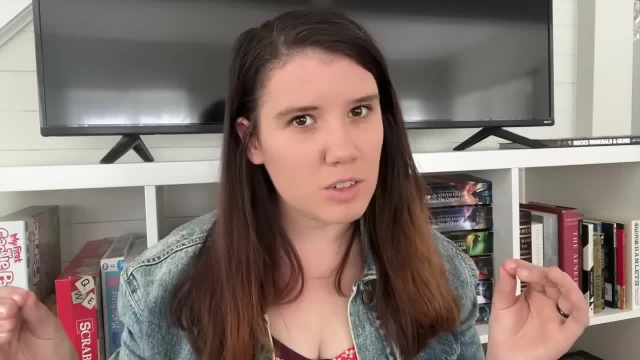 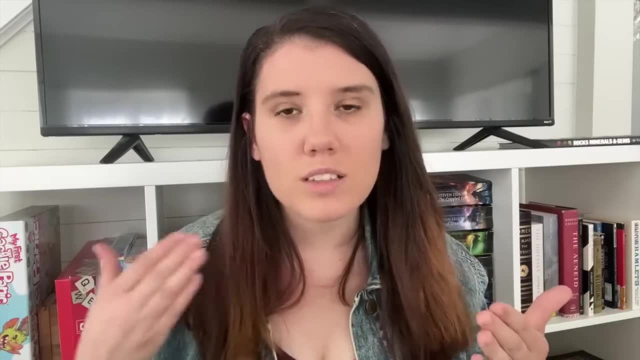 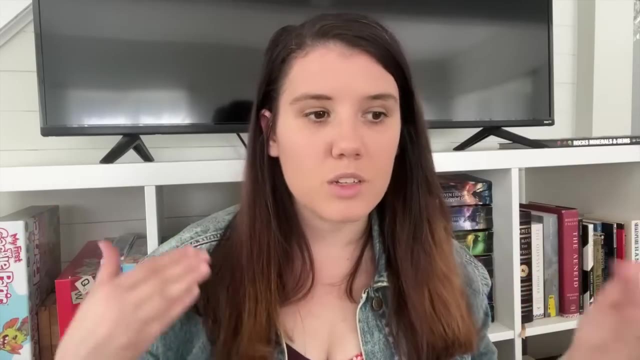 And that's kind of the point for crackpots. A crackpot does not want to do physics. A crackpot wants to be a famous physicist. They want the world to know their name. When you say Newton, when you say Einstein, 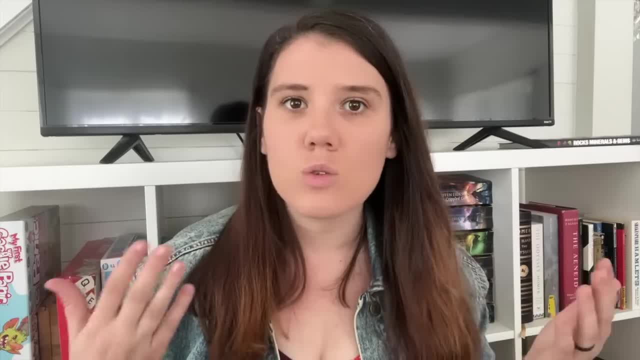 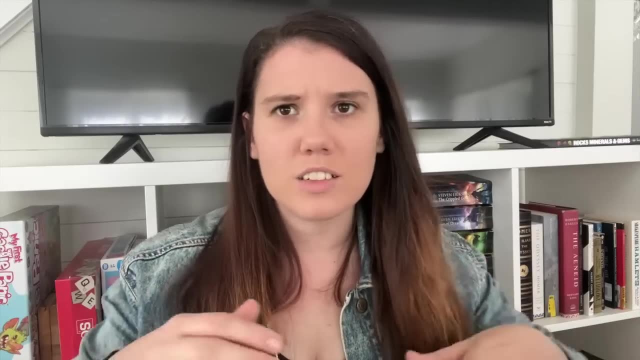 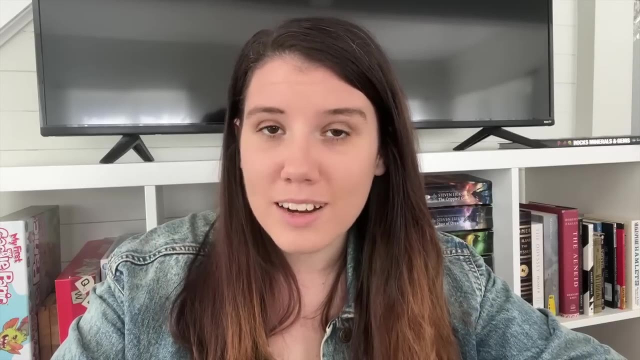 the way Einstein is like a literal colloquialism for intelligence. that's what they want their name to be, So they would never waste their time looking at a small problem And, if anything, if I ever got a crackpot email, that was like solving a small problem. 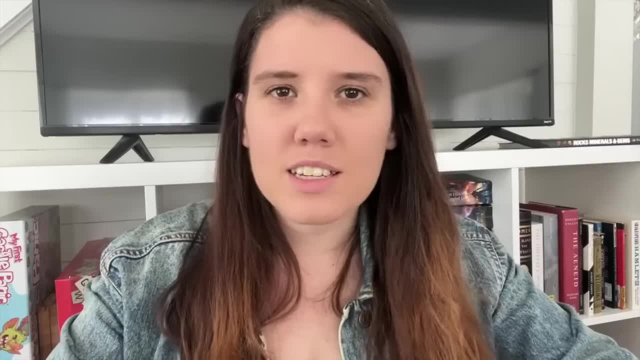 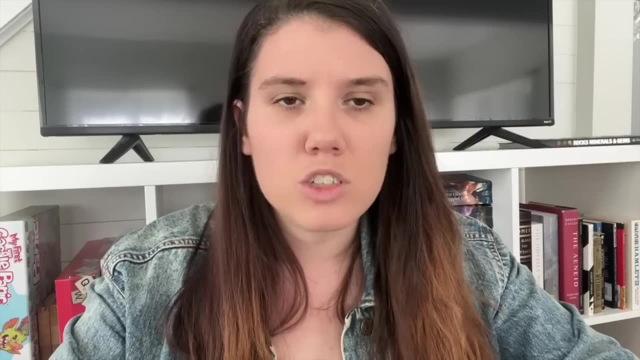 I would read it. I would love to see it Like I want to see. astrophysicists don't take into account granular sorting when they model planetary formation, which means they have two, two times as many planet outputs as they should. 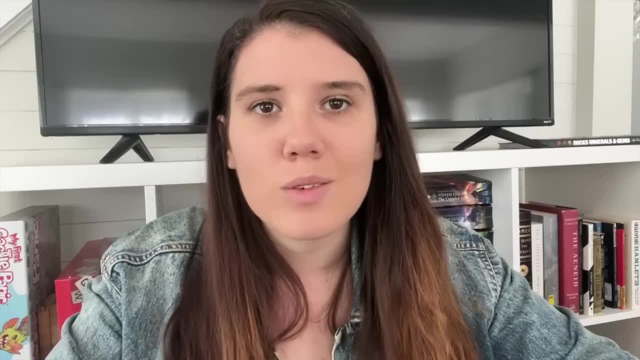 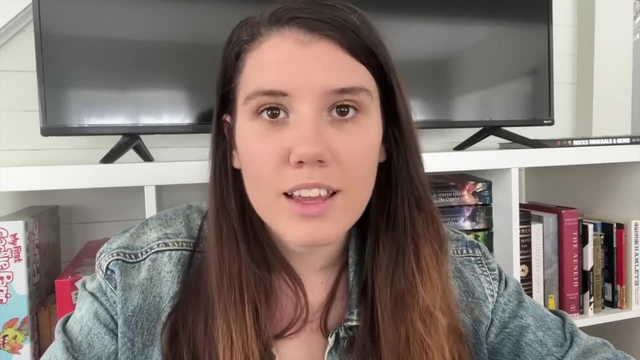 Like what a small, beautiful little problem to solve. I would love to see it. I would love to see a crackpot just be like. here's my method of laser ablation. That's three times as fast as any other current method. 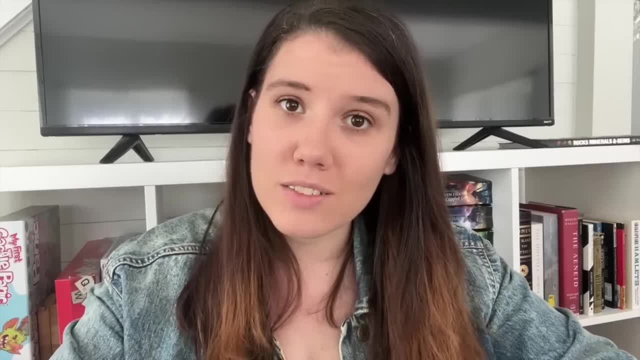 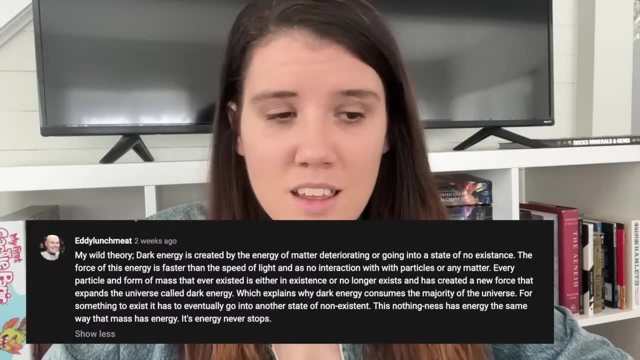 But no, it's always going to be like: here's why relativity is not real. Here's why the speed of light is actually 2c. Got them. So what would an observer see if they were near the galactic center? 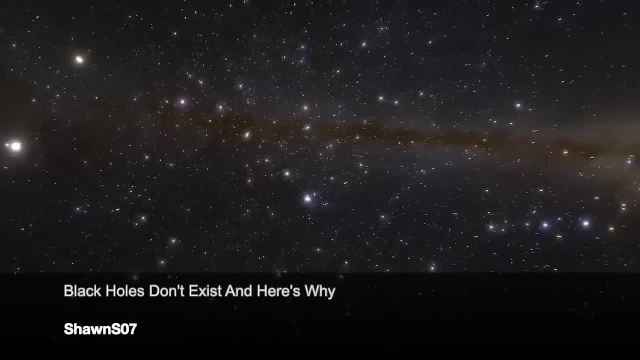 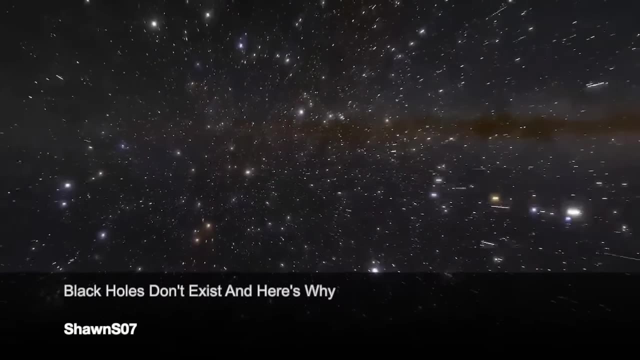 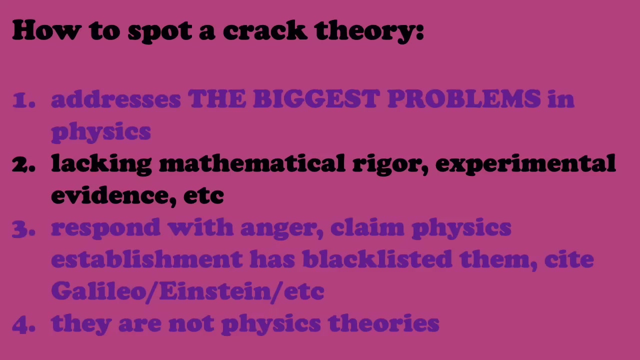 Well, that's misleading, because there is no valid XYZ coordinate that an observer on earth can attribute to the center of our own galaxy, because space time itself is traveling at a higher momentum there. The second thing is, if you do get past the title of, like my theory, theory of everything. 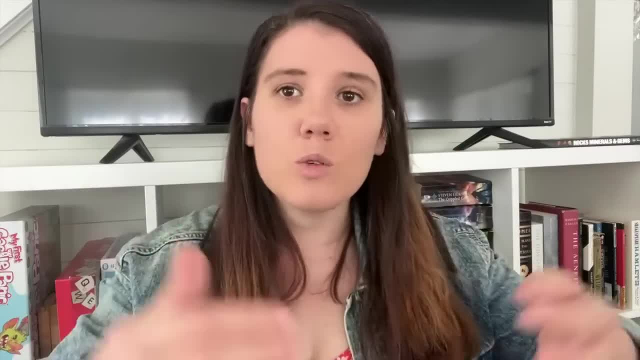 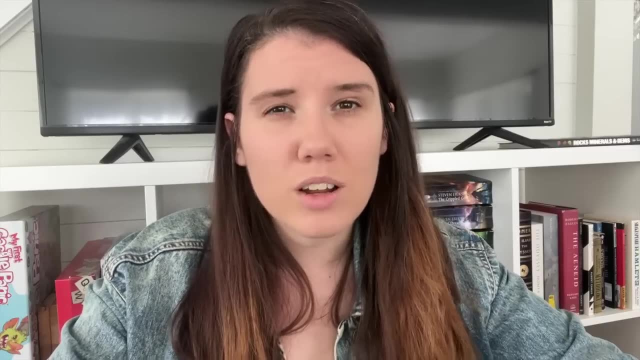 and you open that PDF, you will find no physics at all. There's no math because a crackpot doesn't have physics training. They don't understand math. They don't understand what a physics project looks like. You won't see any math. 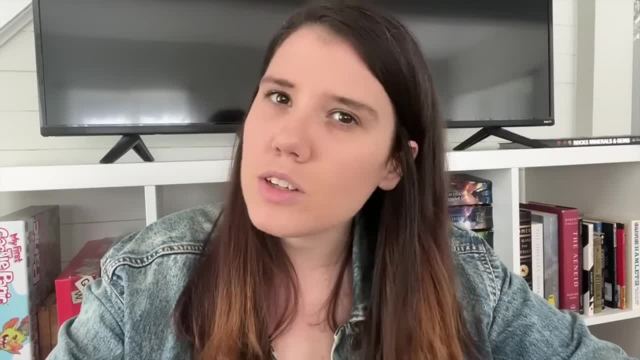 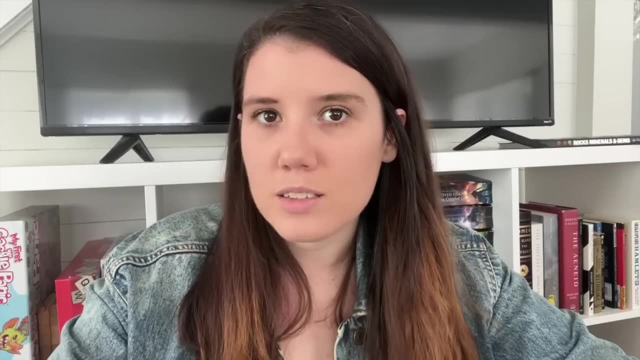 And for this I kind of blame science communication. Like if you give a public talk on quantum mechanics, you can't send a text message two days before to be like: Hey guys, make sure you you're up on your field theory before you. 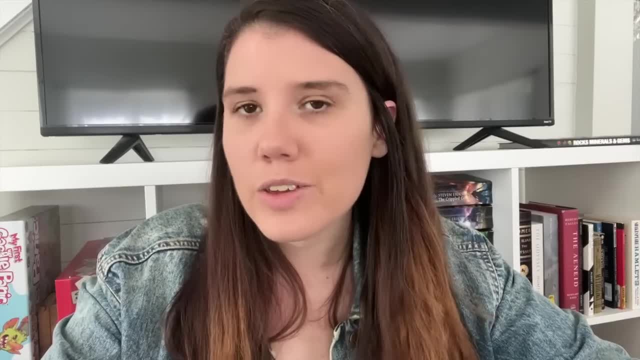 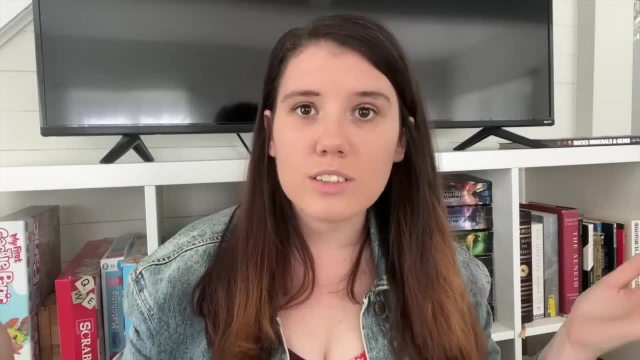 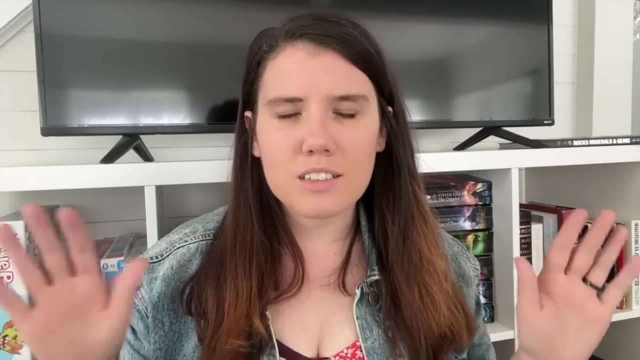 come to my public lecture on quantum mechanics. You can't do math in a public lecture, So what do you do? You come up with stories, with thought experiments, with cool little diagrams and you're like: let me explain the theory to you. But that theory is not the diagrams. 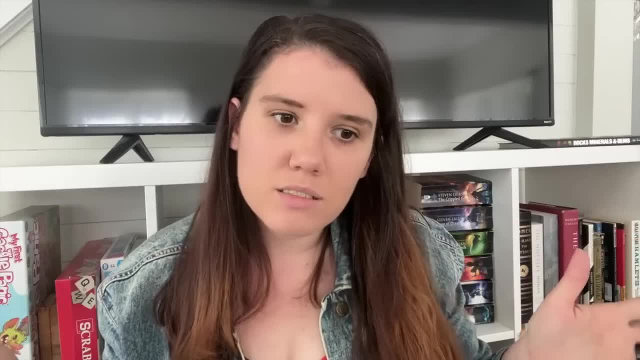 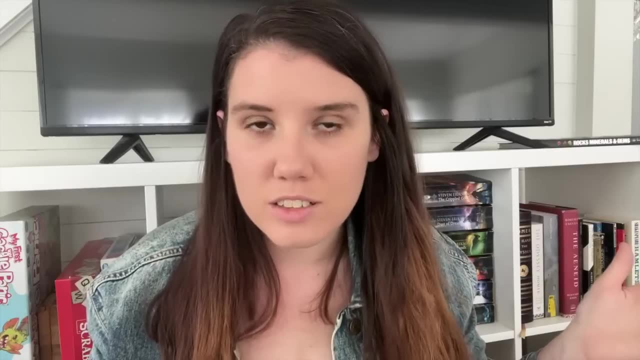 It's not. the cute little stories like Schrodinger's cat is not the proof of the uncertainty principle. It's not the derivation of this uncertainty principle. It's not the derivation of this uncertainty principle. Schrodinger's cat is the joke. 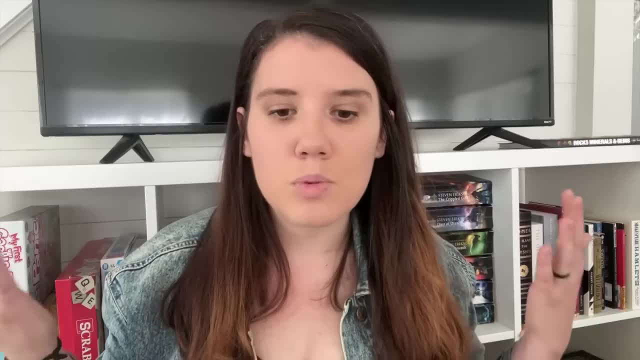 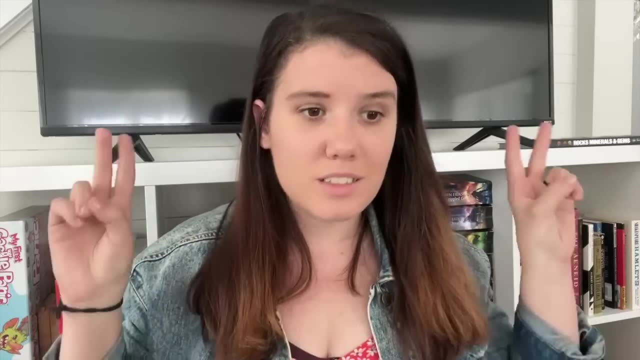 It's a story. It's a little funny thing to say, to point, to poke at like the absurdity of quantum mechanics, but a crackpot will write a theory where they disprove Schrodinger's. I got to stop. They will disprove Schrodinger's cat. 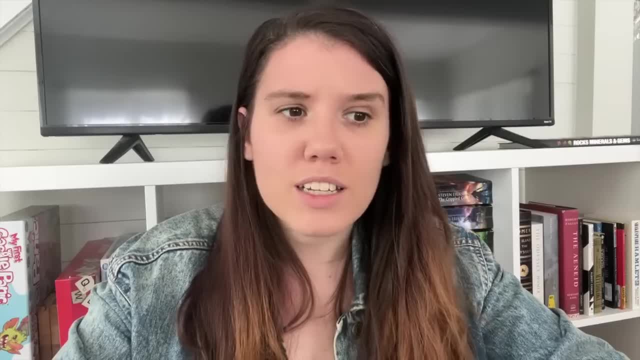 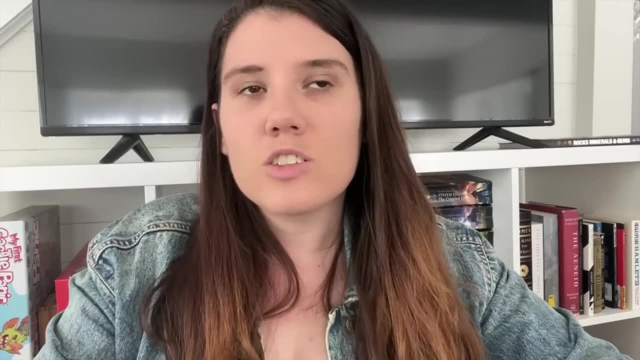 which is not what quantum mechanics is, And they will just write a cute little story about how you can put a camera on the box and tell if the cat's alive. Therefore, quantum mechanics is wrong And it's just like that's Schrodinger's cat. 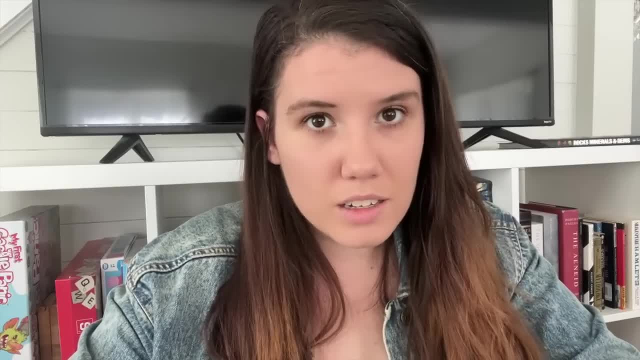 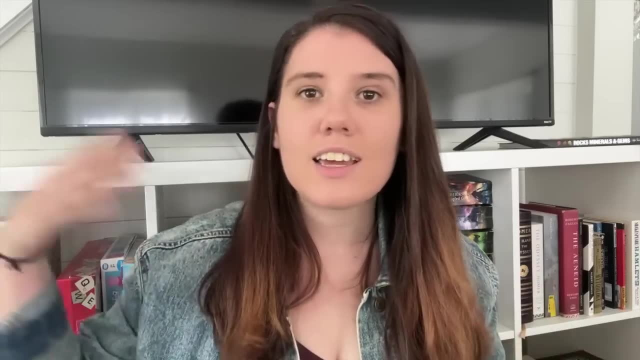 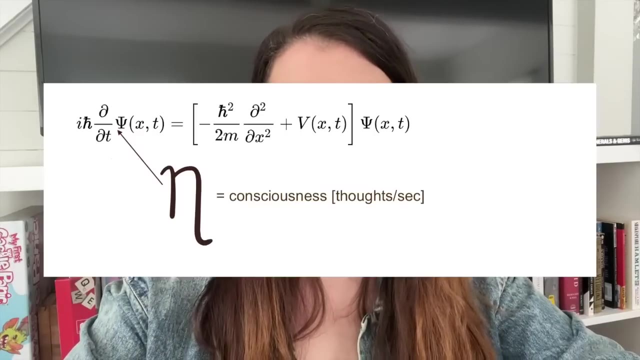 Isn't the theory. So when you open a crackpot theory, you will never see a derivation, You will never see correct math. Crackpots are fond of, just like taking an equation, like the Schrodinger equation, and just like sticking in a little constant. being like this is the new, and new is for consciousness in the wave. 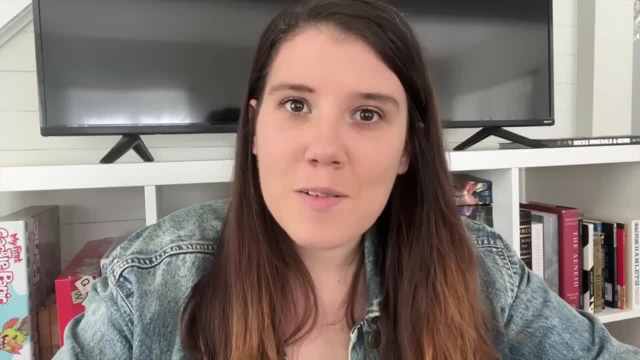 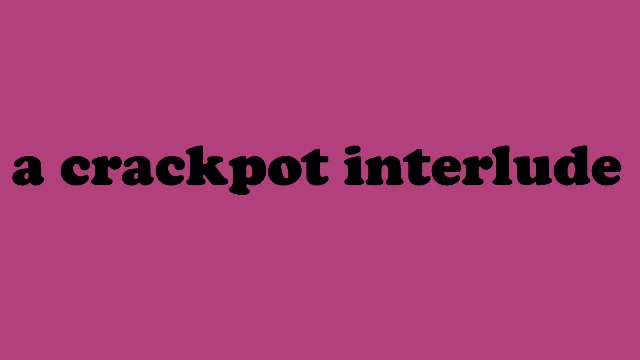 And I've added it and it's like: OK, but what are the units? What are the units of consciousness? Isn't that going to mess up Your Equation? They don't know, They don't care. As the boys, equations apply to all matter. 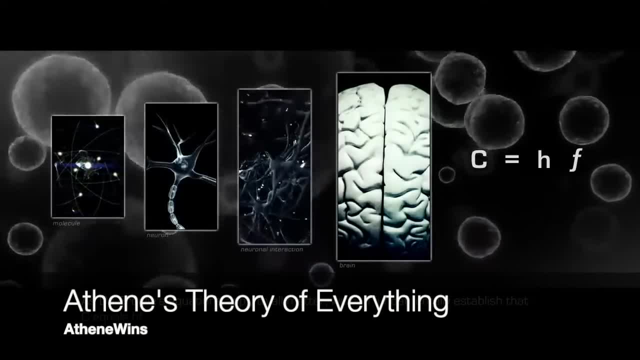 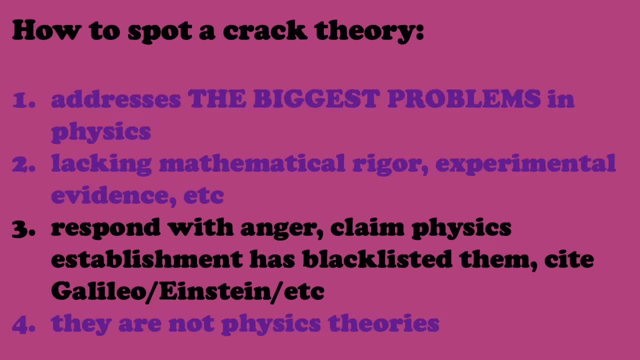 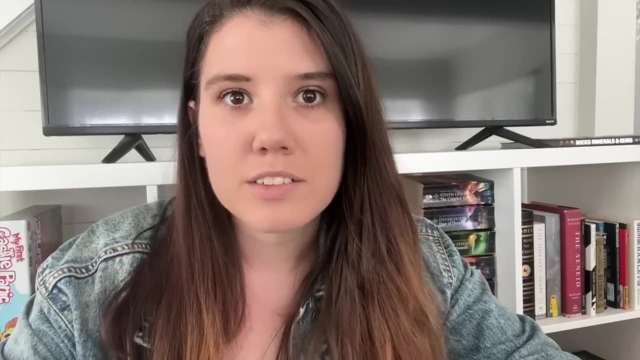 we can fundamentally establish that C equals HF, where C stands for consciousness, H for the constant of Planck and F for frequency. That leads me to the third thing that tells me this email is actually a crackpot theory of physics. Crackpots are incredibly. 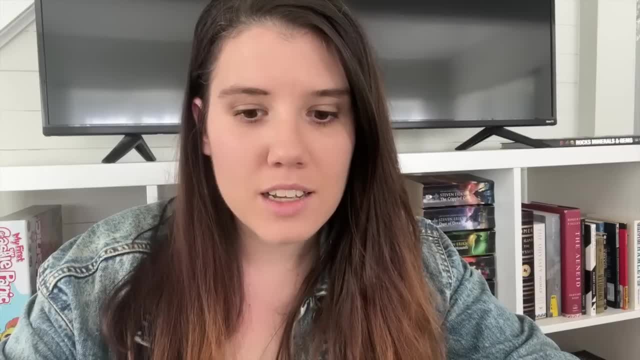 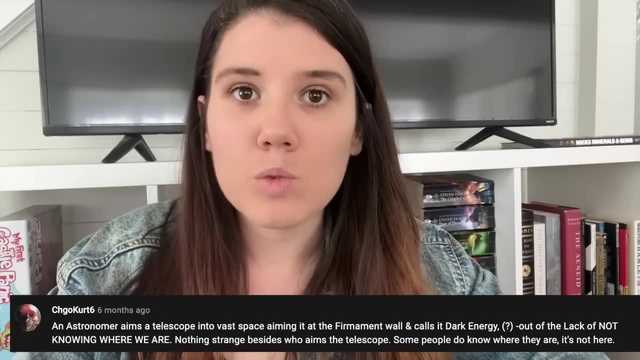 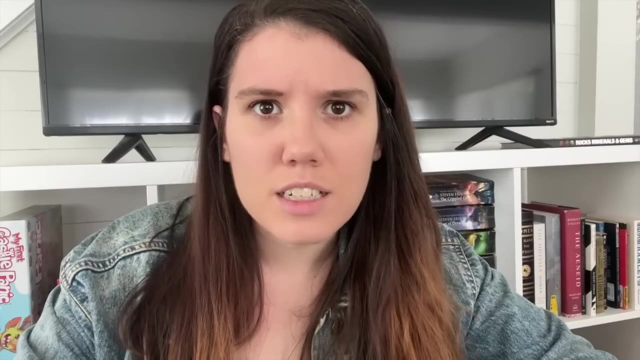 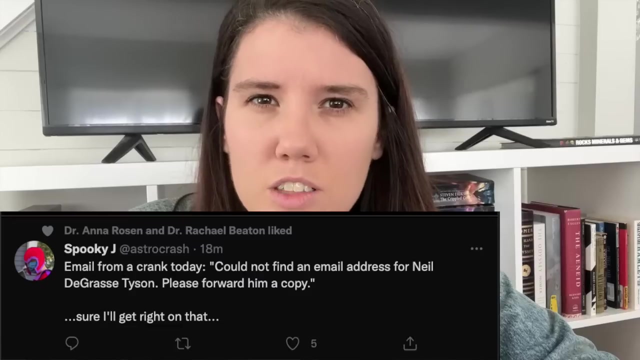 Angry at the physics community. Crackpots will send you emails in all caps with random words in bold and in red and say things like: the physics establishment will regret not listening to me. If this email doesn't reach Neil deGrasse Tyson in 72 hours, you'll be sorry. 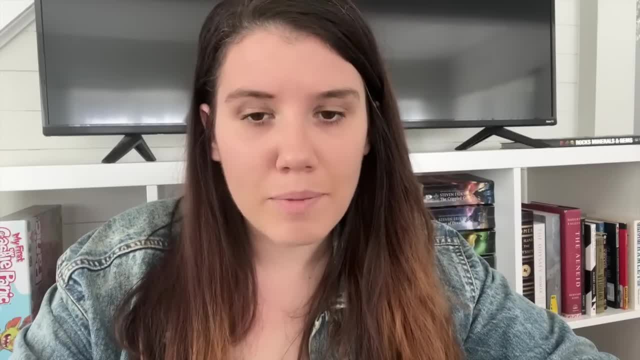 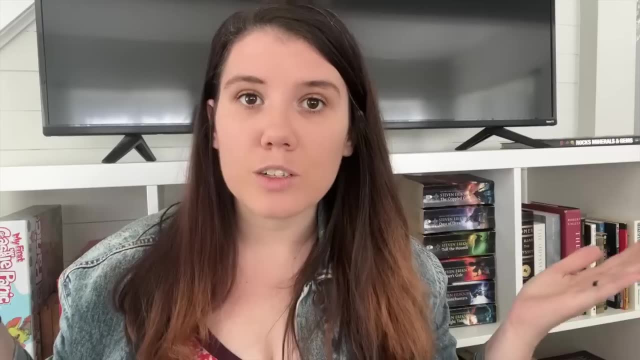 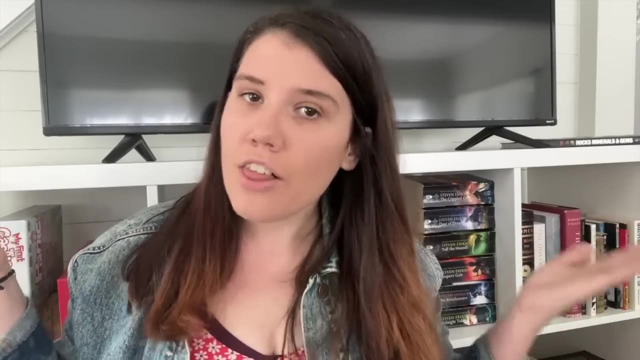 Like you, you have ignored me for the last time And honestly, bros, it's a little terrifying, because physicists usually work at public universities. It's like you can Google your local university, go to their physics department and find out what building that physicist is going to be in all day. 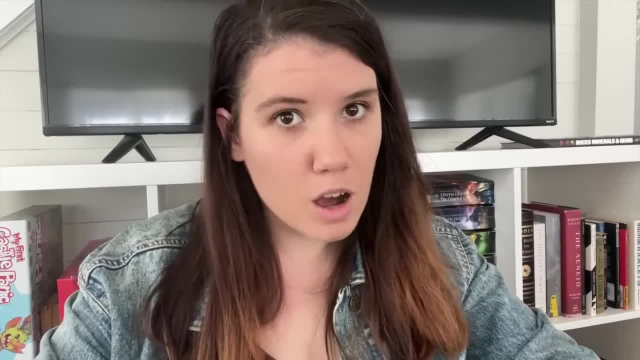 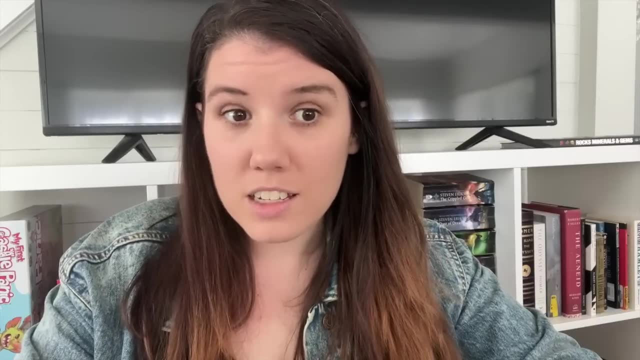 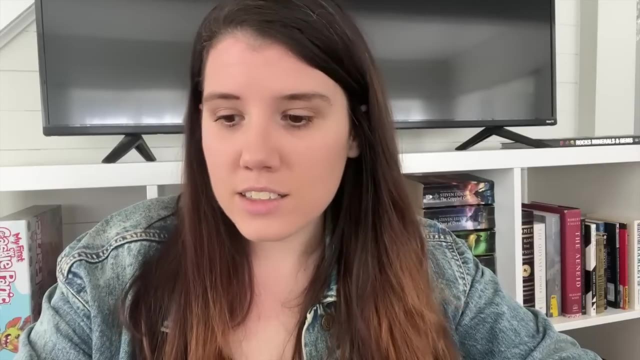 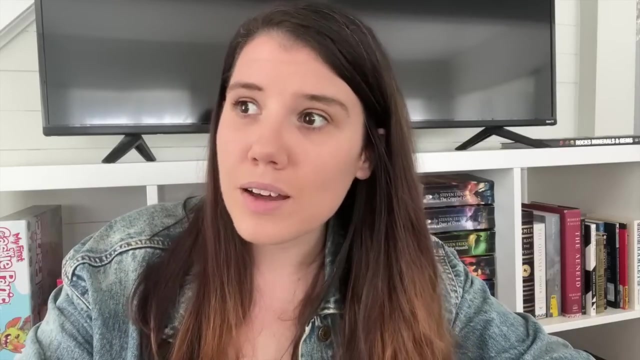 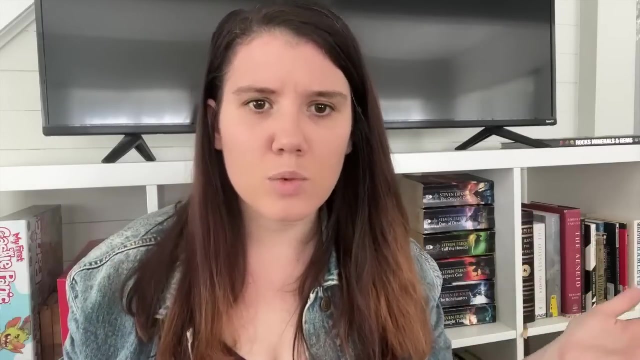 Find out where she's teaching her classes, where her office is, when her office hours are. So the reason I'm never responding to a crackpot email is because they are so, So Angry and it's scary and like it's all fun and games like ha ha ha the. these people don't understand physics. but think about how delusional you have to be. like you open a physics textbook and you're like: I don't understand a word of this. like a normal response would be like: of course I don't understand this advanced topic. 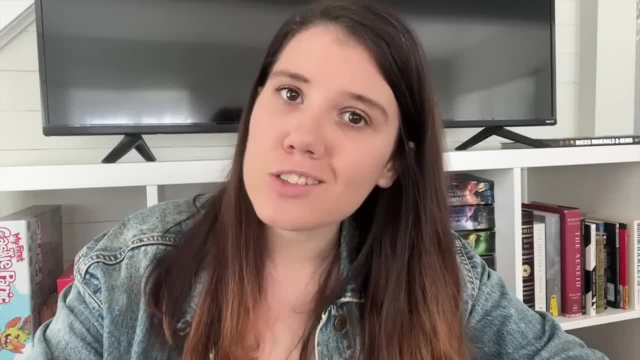 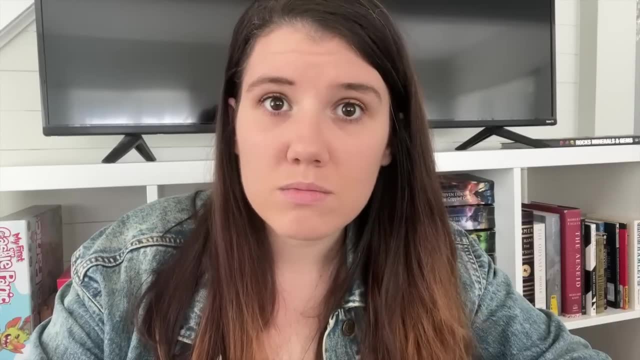 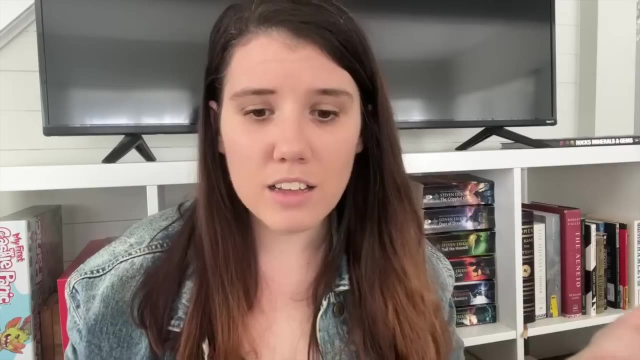 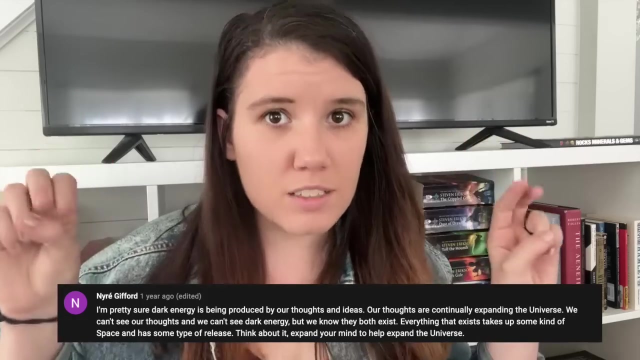 I haven't had physics since high school. Maybe I should start with something a little easier. But the physics Crackpot had that experience and was like: well, all physics is wrong, I'm right, I will be Albert Einstein. And instead of taking a class, instead of learning math, they spent three years independently researching their theory and writing it up. 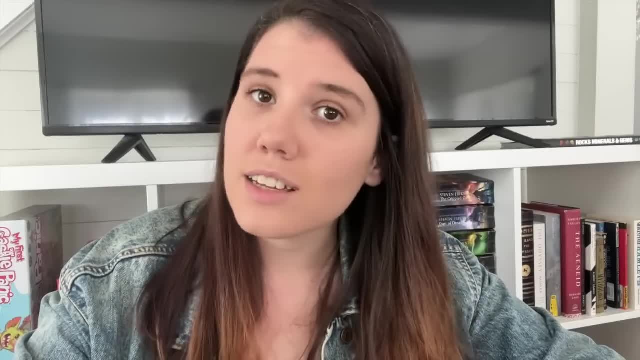 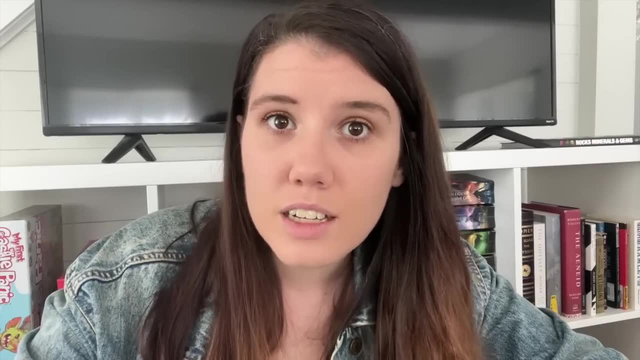 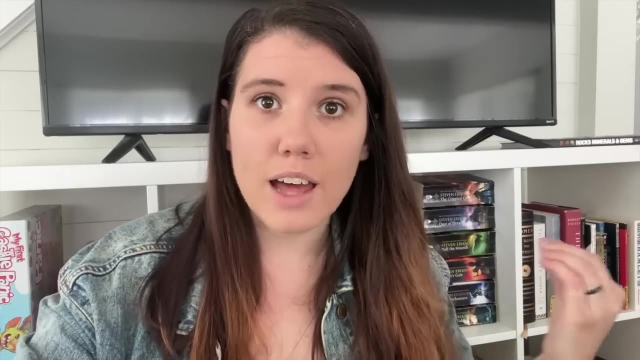 And they sent it to physicists, and physicists respond like it's a joke because it's obviously crank, Like there's nothing there, There's no physics there. And these people get very angry, Like I have worked on this theory for three years and you laugh at me. 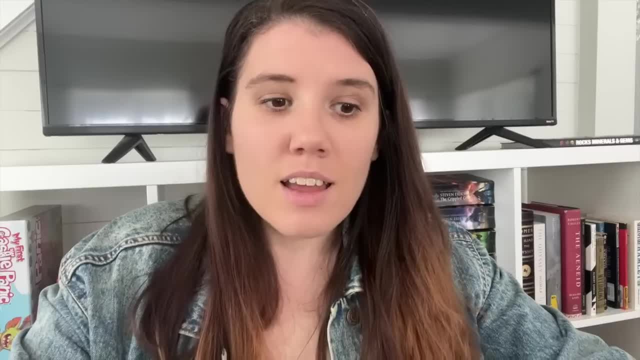 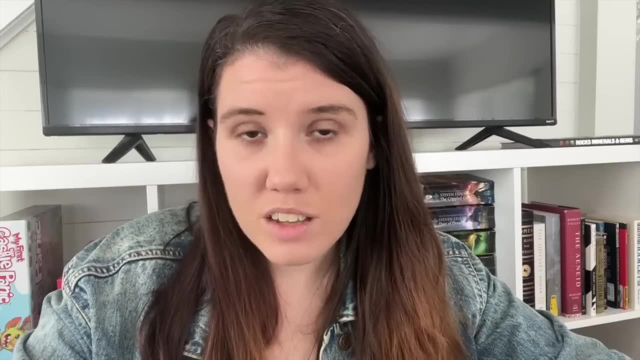 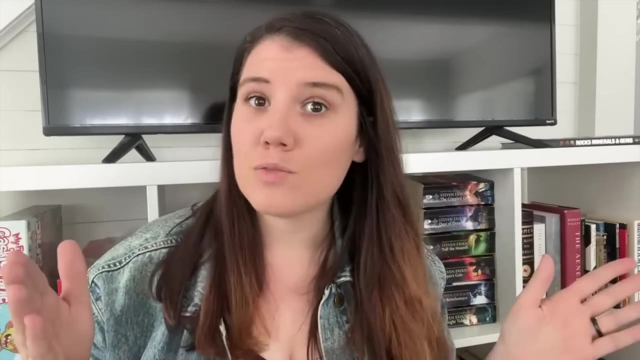 I am going to change the world And this is terrifying. The American Physical Society has conference every year and every year they have a crackpot session. If you pay your dues and you are an active member of APS, You can go to the conference and you can present. 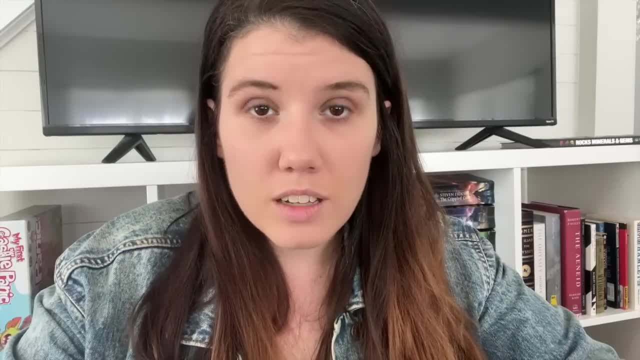 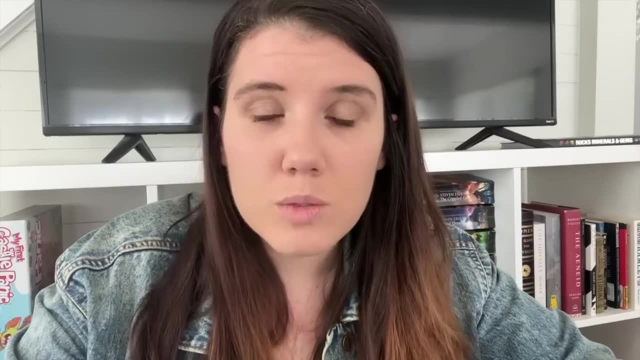 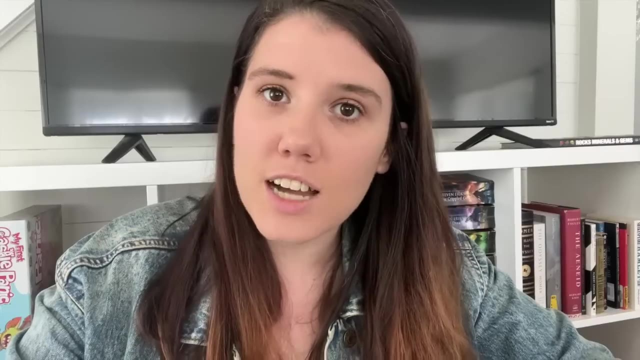 And you know why. In 1952, after his paper on how the electrons don't exist was rejected, a man got on a bus, went to New York, went to the APS office and shot the first person he saw. The first person he saw was 20 year old Eileen Fahey, and she died. 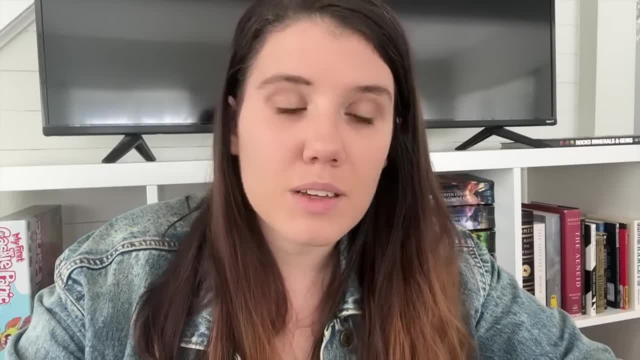 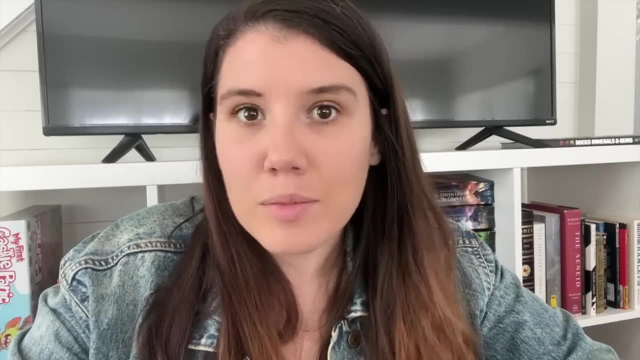 And so now, if you pay your dues, you can go and you can present your physics, because the APS doesn't want something like that to happen again. Okay, But it happened, and crackpots are scary. That's why no one's responding to your emails. 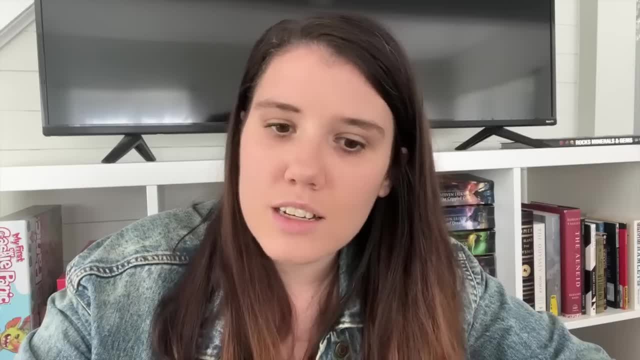 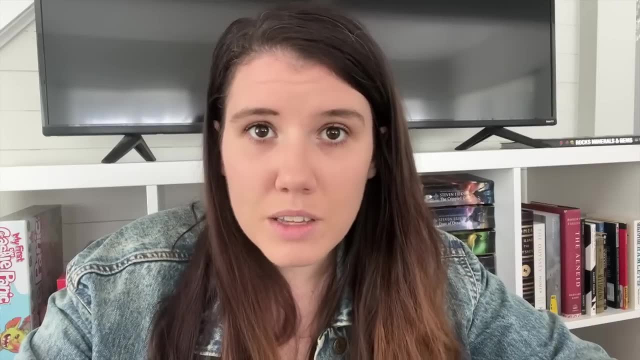 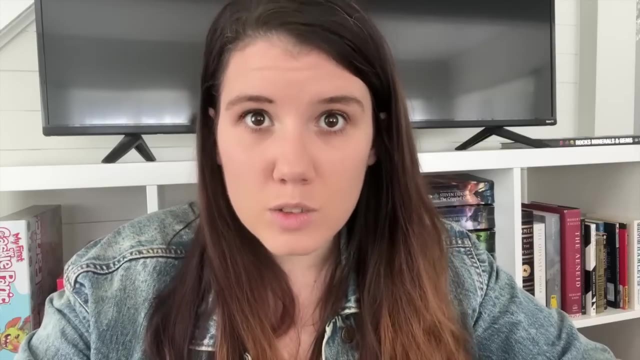 The idea that a random person just sitting in their bedroom could come up with a better theory than the literal thousands of people who work on this every day and have for hundreds of years is delusional. And when you talk about this with people who aren't physicists, they're like: well what? 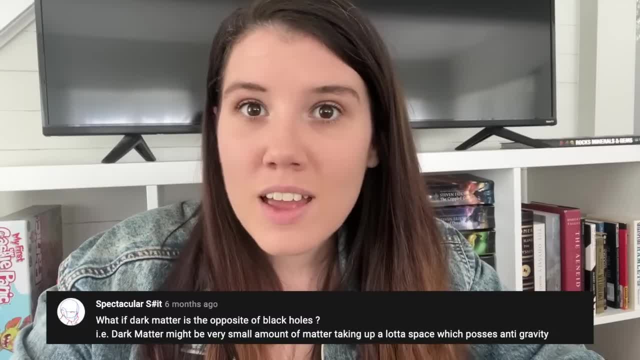 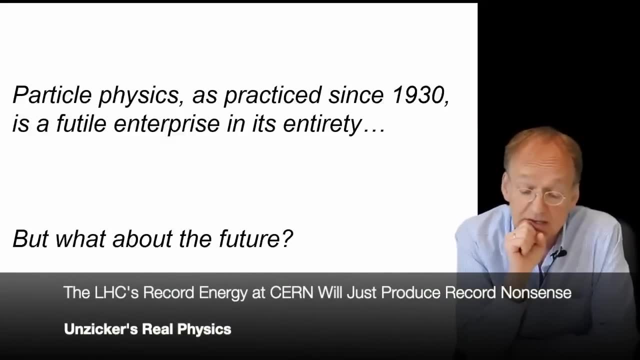 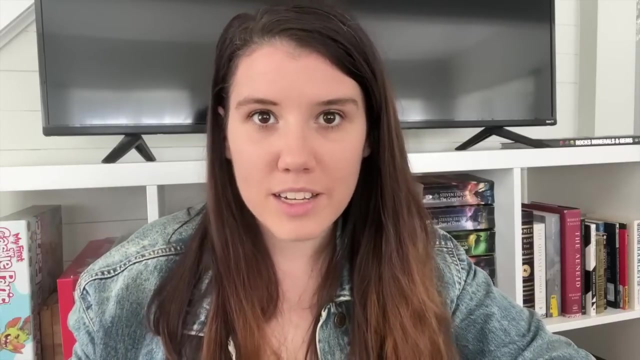 if they're right? What if they're right? And that's the fourth thing. So my conclusion is: particle physics, as practiced since 1930, is an entirely futile enterprise. And that's the fourth thing about crackpots: They will never be right because they have no physics training. 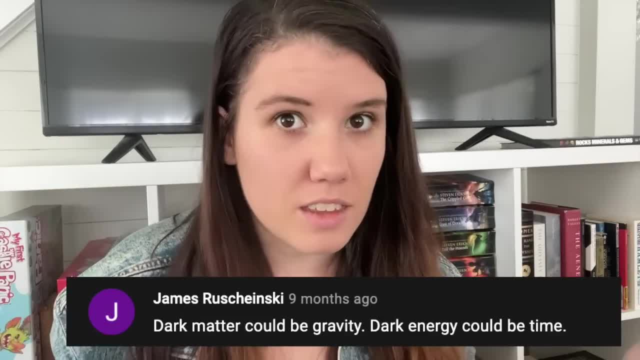 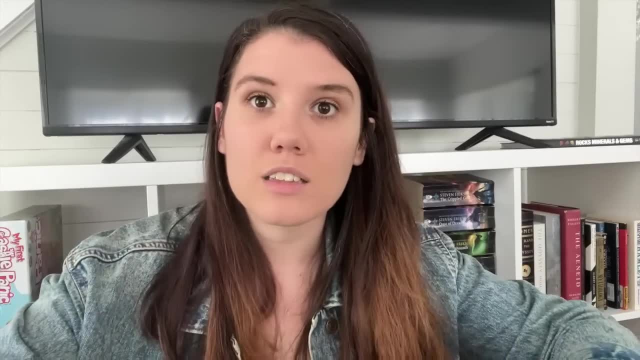 The theories they send are not physics Theories in any sense of the word. Most people do not work at like the forefront of science And so they're like: what if they're right? What if a crackpot is right? What if they're right? 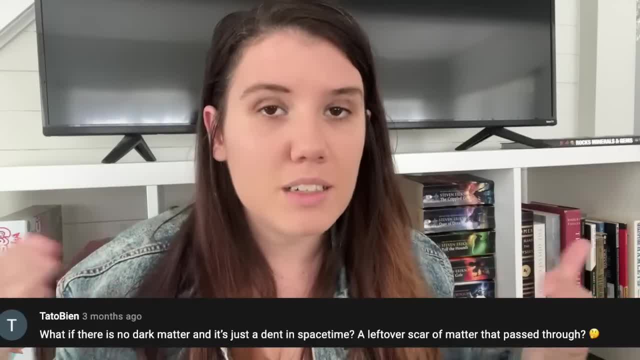 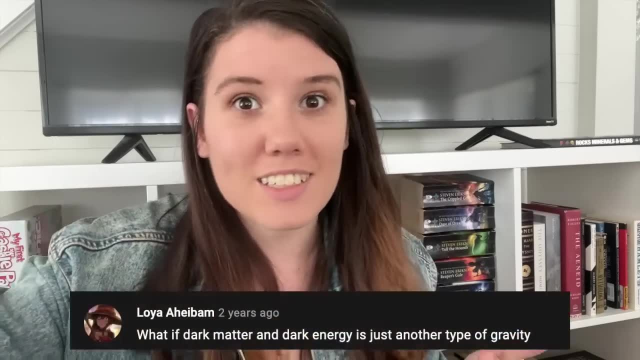 And it's hard to explain. Like it's impossible for them to be right because they are not doing physics at all. Like they could never be right because they don't even take the step to have a physics idea. So, in classic physicist fashion, I have prepared an illustration, a cute little story. 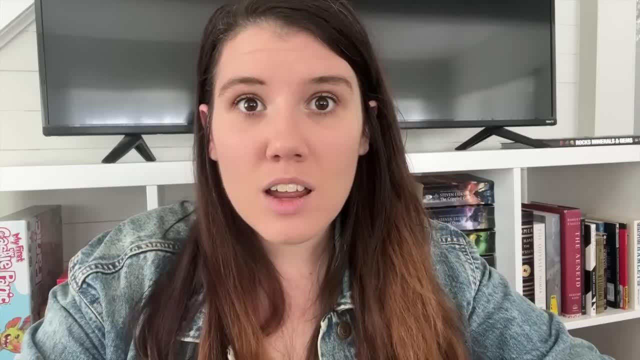 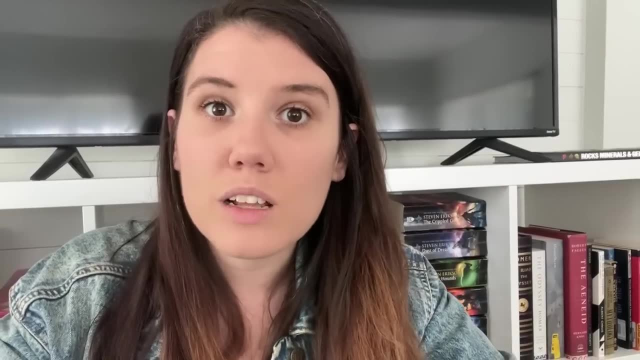 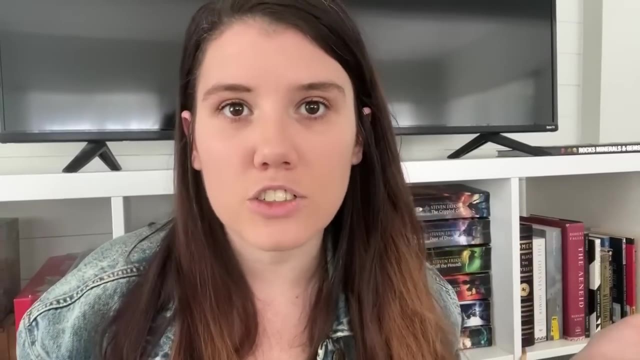 A la Schrodinger's cat to explain to you what it's like to receive a crackpot email. Imagine you work in a restaurant and you have been head chef for 12 years. People love your food, People love your recipes. One day before dinner rush, someone just busts into your kitchen and he says you're part. 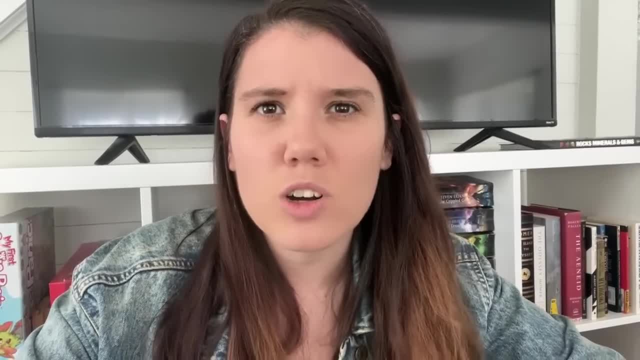 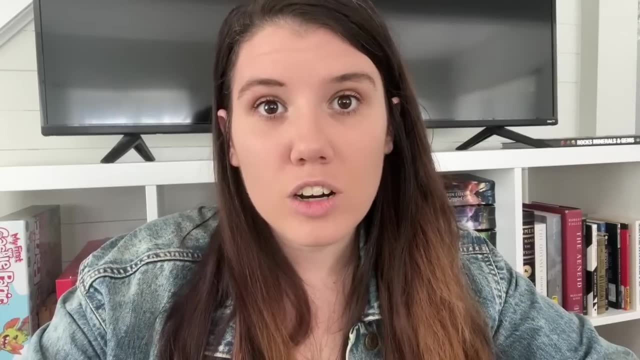 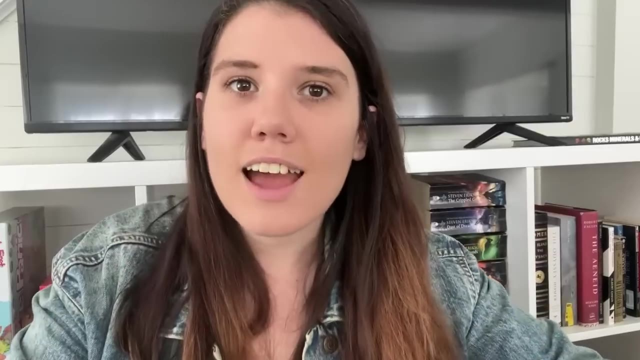 of the chef establishment. You don't know what a recipe is. You're all wrong. I am the best chef in the world. I make the best recipes. You're garbage. And they just throw a takeout box like down in front of you on like your bench. 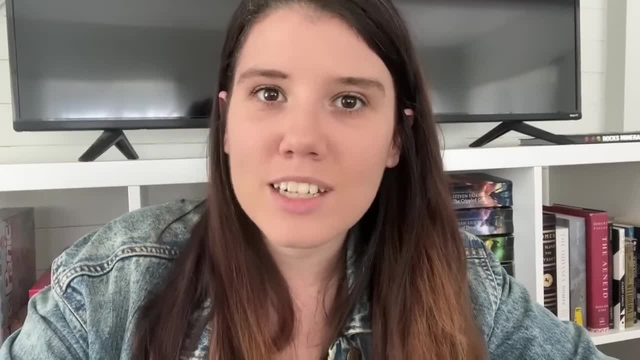 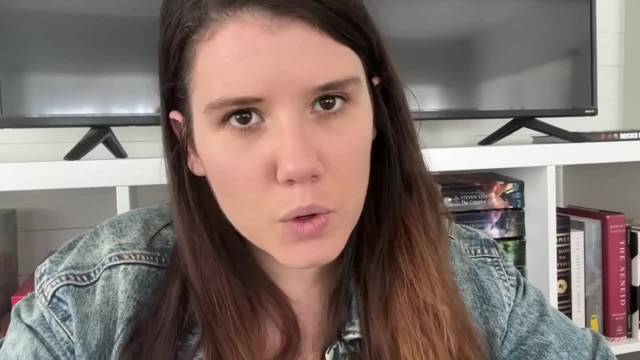 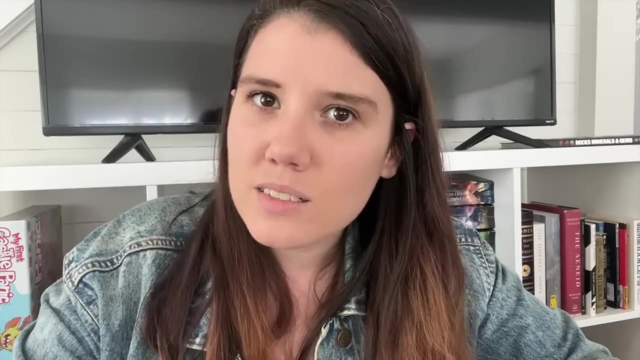 How do you feel? You're pissed right Like: how dare this person come into your successful restaurant and call you garbage? You're mad, right, That's incredibly rude, but you're curious. You're curious, So you open the takeout box and it's Play-Doh. 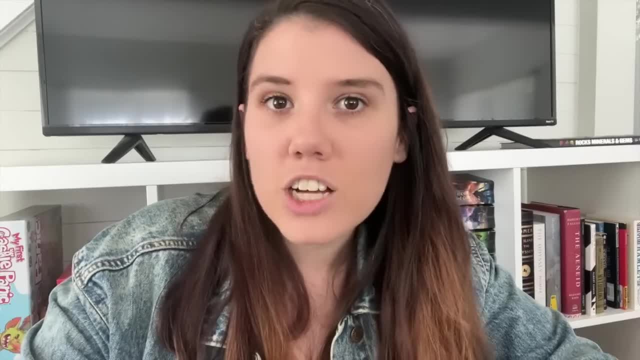 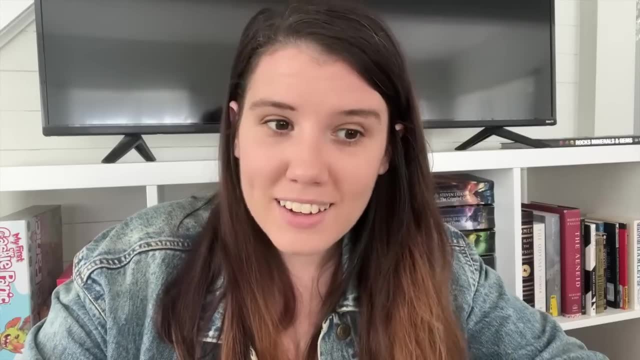 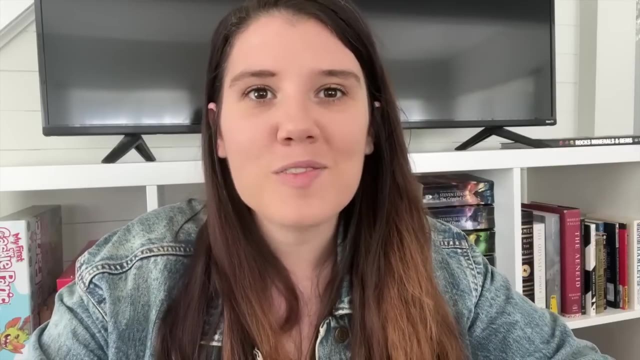 Is Play-Doh arranged to look like a pop. What does it look like? Look exactly like Pasta, the way like a child, a three year old, would make. So you laugh because you think it's a joke. This man came in all pretending to be angry and he's like: look at my recipe. 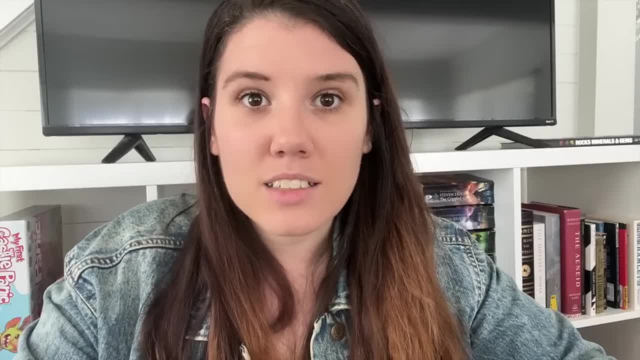 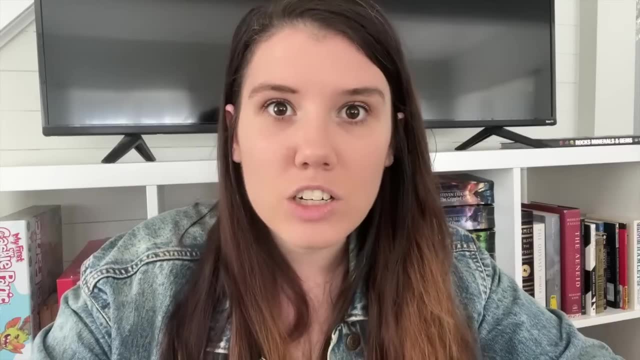 It's the best And it's not even a recipe, It's Play-Doh. How funny. And when you're laughing he looks at you and you see that crazy, like delusional, like empty eyes, And he starts screaming. 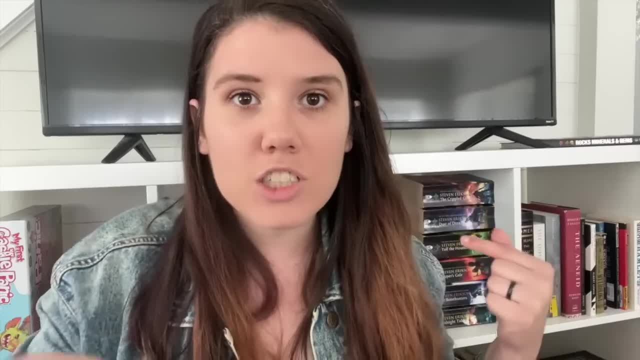 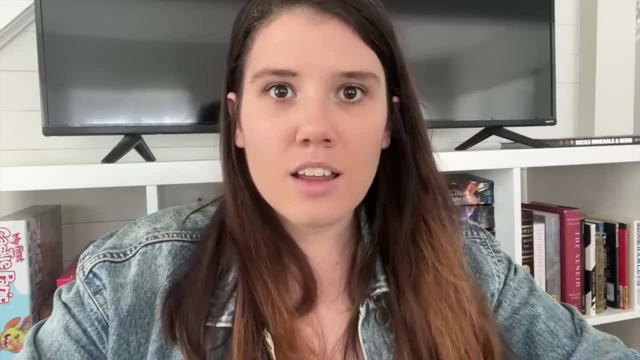 How dare you laugh at me? I've been working on this recipe for three years. I don't know what's wrong with me. I will change the world. I am the Bobby Flay of 2022.. How dare you? And now you're scared. 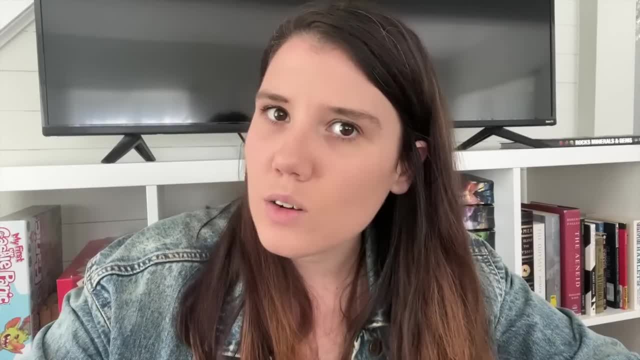 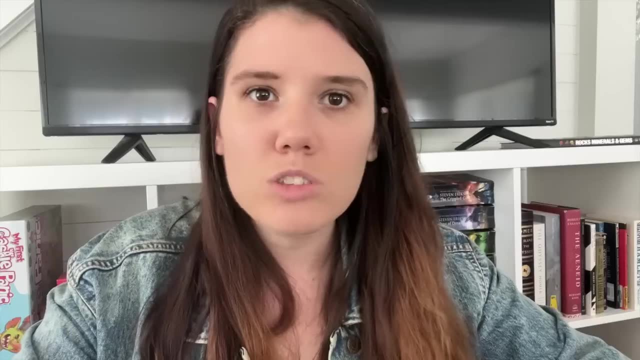 right, Because this man thinks this is food, but it's Play-Doh. It's not food. How did he work on this for three years? He never Googled what is a recipe, What is food. He didn't go to a restaurant. 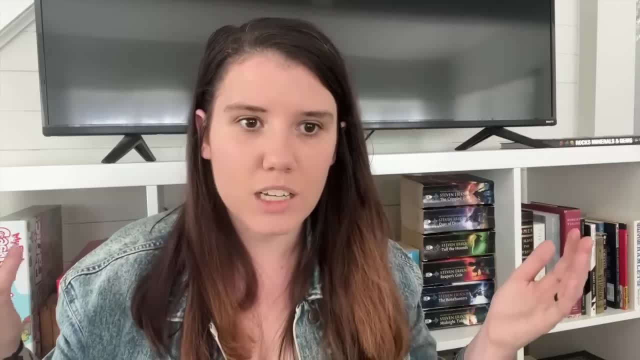 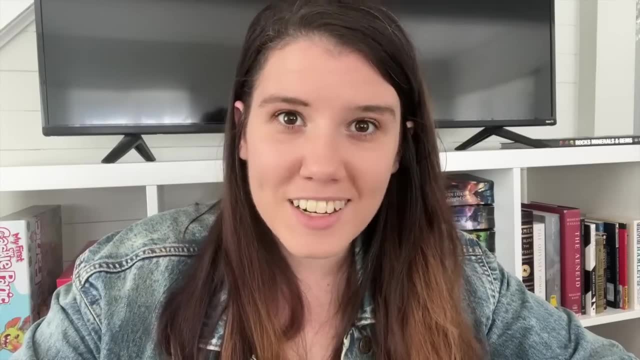 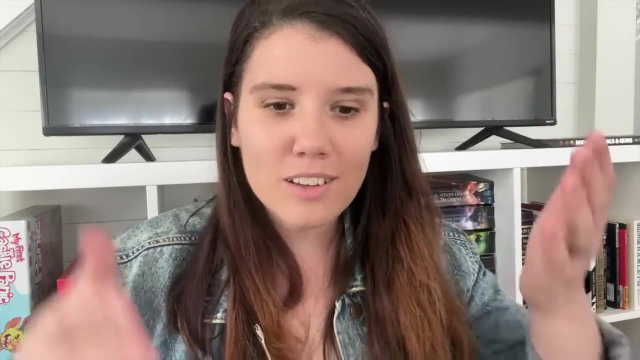 to test other people's food. He's been working on this for three years and now he's in your kitchen. He knows where you are. It's scary. And now imagine people are like: well, what if he's right? What if he's right? He's been working on it for so long. Maybe that is the best recipe And you're. 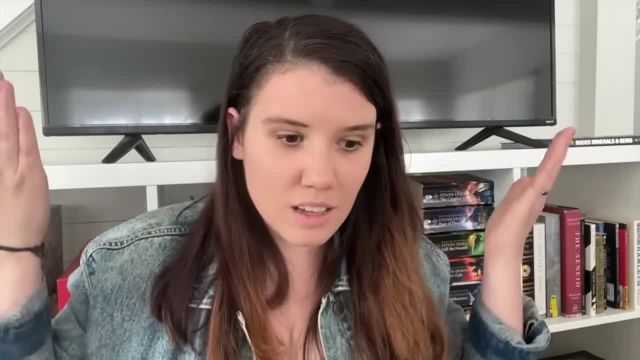 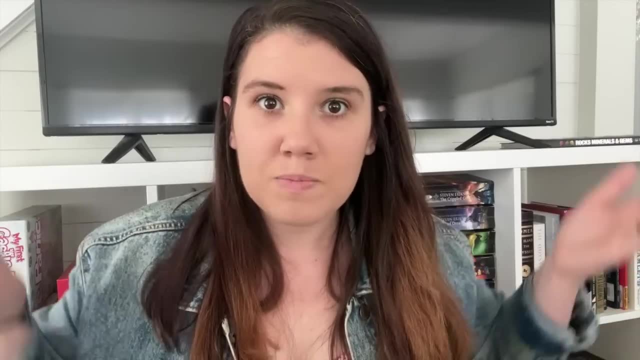 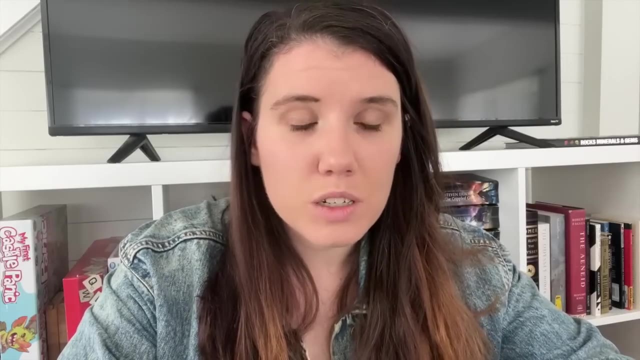 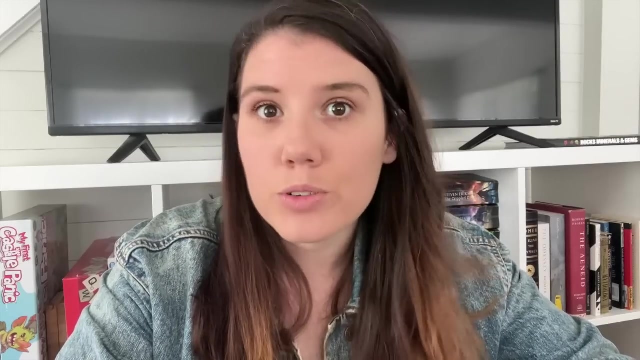 like. it's not even food. It's Play-Doh. It's not food. He didn't do the basic. He's not speaking my language. I can't eat this. Crackpots have no conception of how physics works And they take rejection as evidence that their theory is correct, because they're delusional. 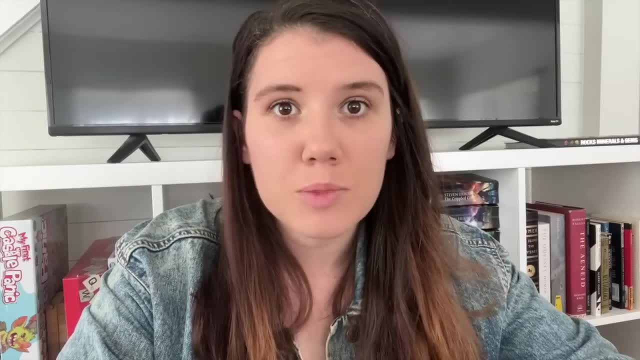 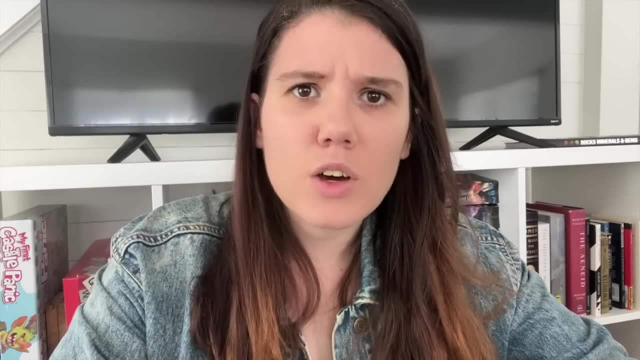 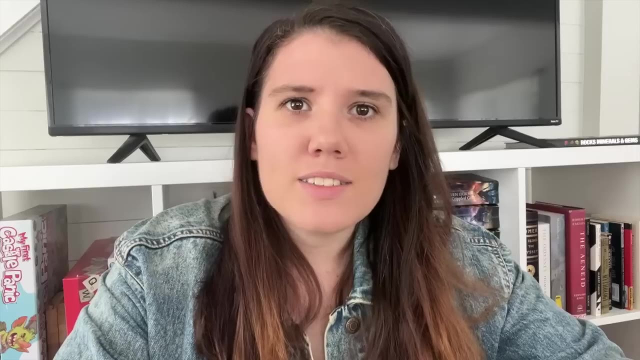 They think like: see, it just proves that the physics establishment is afraid of me. They'll cite Galileo and say: just like Galileo was proven right, I will be proved proven right. And it's like everyone believed Galileo. What are you talking about? They'll be like Einstein was bad. 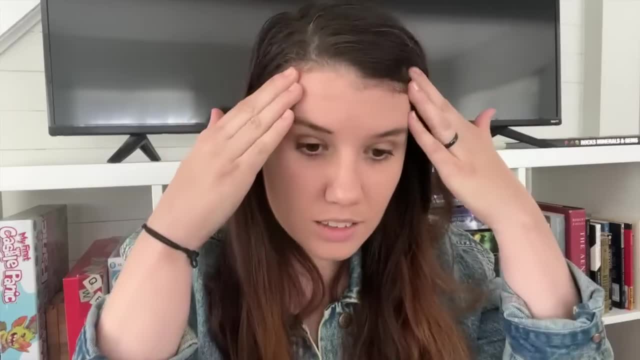 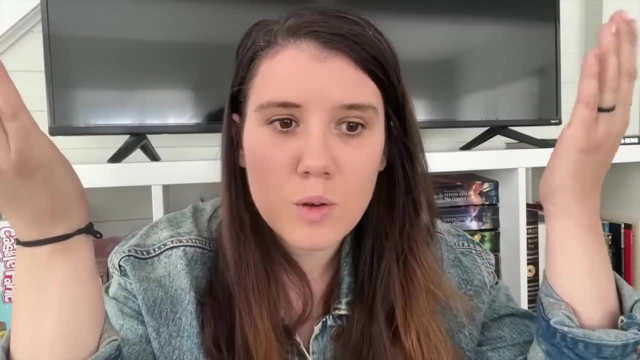 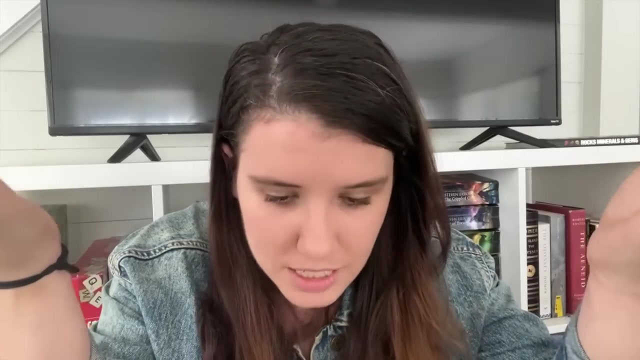 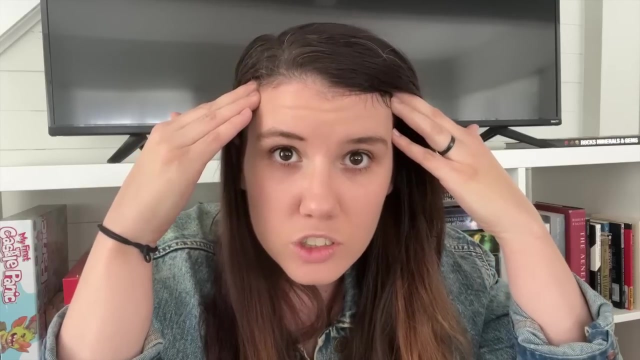 at math. He was a patent clerk, And it's just like what. Of course, Einstein was brilliant at math. He's like the most famous theoretical physicist. He was a patent clerk, but he was also a professor. He was also trained in physics. Like people believed Galileo, but he pissed off the church And so